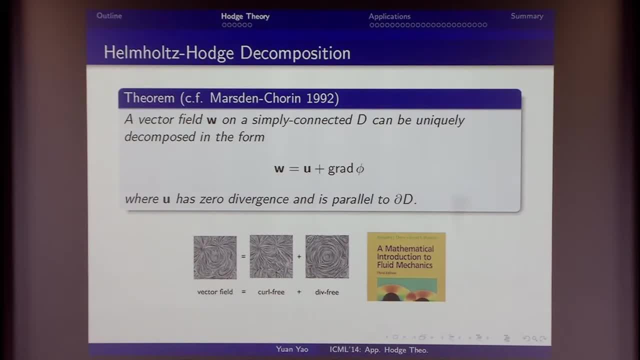 of today's talk And suppose you might remember in your multi-varied calculus course a theorem like this. This is called Helmholtz decomposition Means given any vector field on a simply connected domain, D, and it can be unique, Basically decomposed in this form, The first line is called divergence-free flow. Basically, 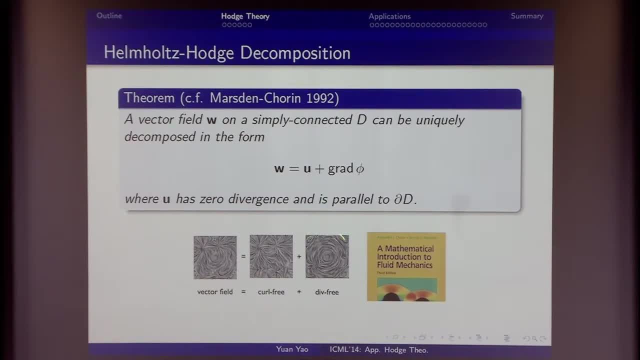 it's a kind of cyclic flow or cyclic vector field. The second is called the gradient field, which basically starting from somewhere and ending with to somewhere, And so this kind looks like a potential gradient. So this decomposition actually happens on the plane with simple connected. 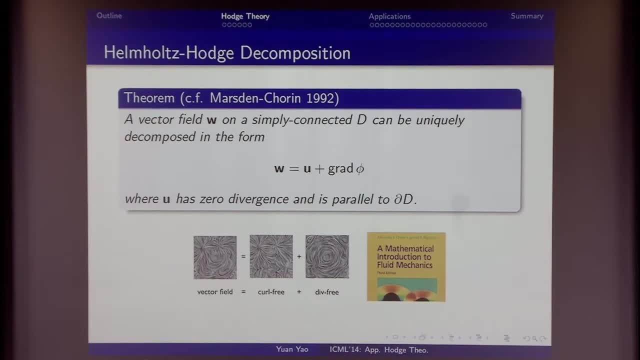 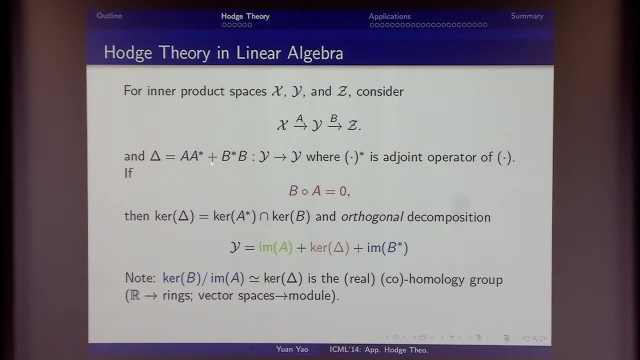 means there's no holes in the domain, And this picture actually coming from Gerald Mastin, who passed a few years ago, and Turing's classic book on fluid mechanics. But you probably wonder what's the essence elements in this Hodge theory. So I just give you one particular picture in terms of linear algebra language. 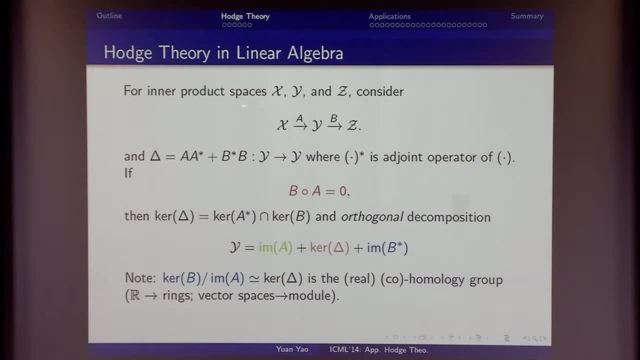 So you don't need to worry about anything beyond linear algebra. Suppose you just have three inner product space- X, Y and Z- and we have two operator or two matrices: A acting from X to Y, B acting from Y to Z. 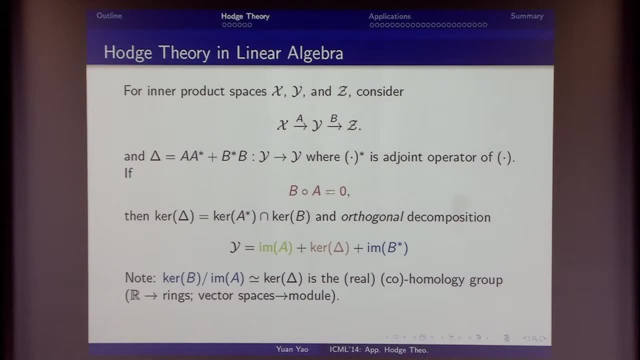 And this composition satisfy this particular rule. the A followed by B must equals to zero. That's the only constraint we are going to use And we can define Laplacian operator like this, acting from Y to Y. Basically, you come, come from this direction, go A adjoint because vector in the product space. 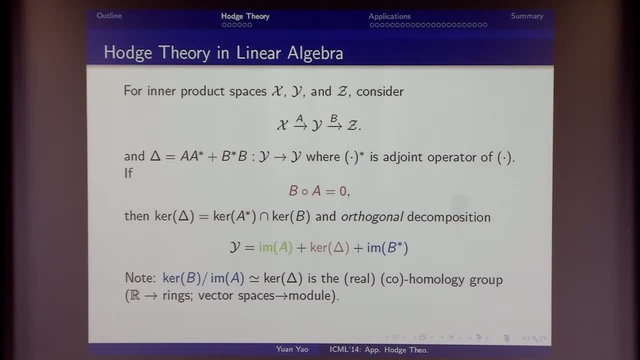 you can always define adjoint operator, So from A adjoint to A and pull back here in another direction, B and B adjoint, then come back. So this kind of abstract Laplacian operator will be defined in this way. So whenever you have this kind of condition, 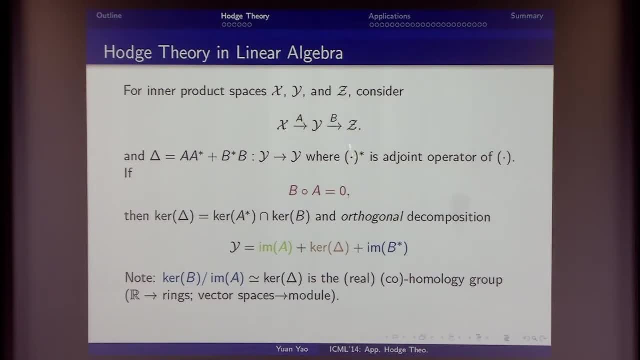 you can show by linear algebra language. the middle inner product space Y always admits this. this orthogonal decomposition- This is canonical, basically image of A plus kernel of this Laplacian operator and the plus image B star. So that's the Hodge decomposition. 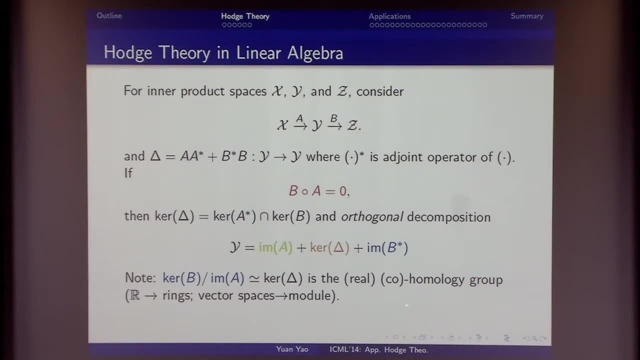 So various kind of language can be associated with this type of decomposition. You can call homology group or cohomology group, depending on what kind of the domain, the field or the module you are going to use to define the vector space and in the product space. 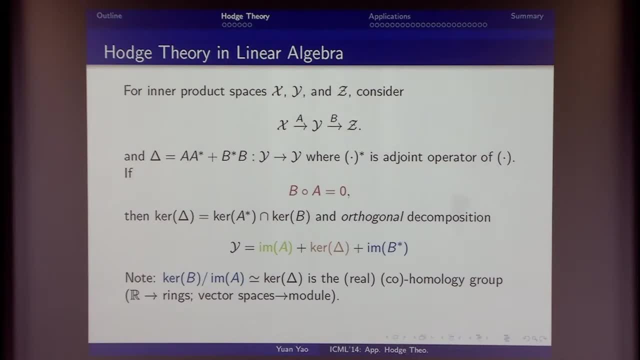 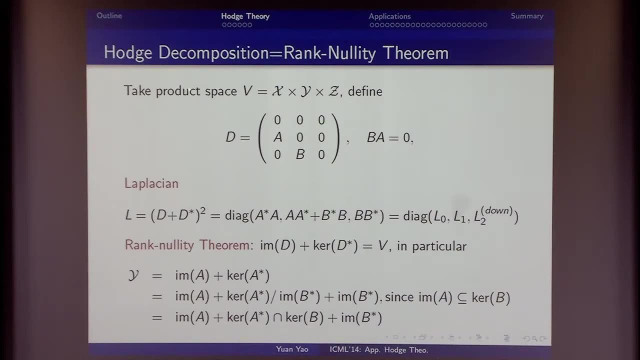 So I won't. yesterday Lei-Heng gave you a very comprehensive list of various name- can be algebraic topology theory names. But here I just give you the one answer: how to prove this simple theorem. So this one turns out to be equivalent to the rank nullity theorem in. 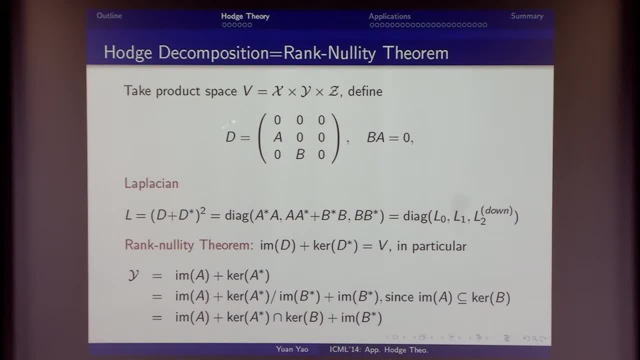 linear algebra You don't need to worry about too much, And this is to use rank nullity theorem to prove the Hodge theory. Basically you can define a big space- take all the X, Y, Z as a product- and a big operator. 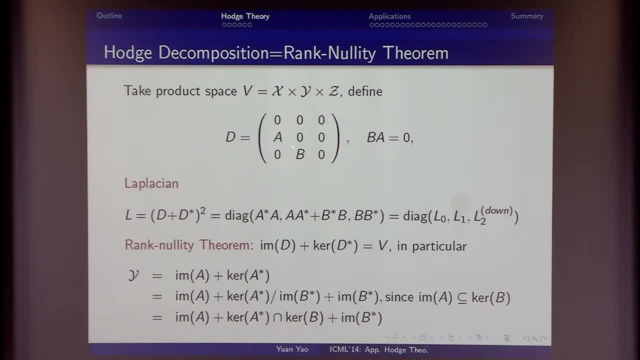 which consists of A and B in the lower diagonal and all the other parts equals to zero. And together with this important constraint of B, followed by A, followed by B, must, vanishes And Laplacian, we can define a high dimensional Laplacian. 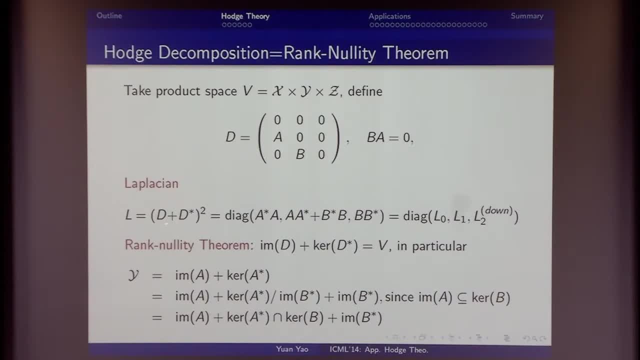 make all this, stack everything together. We take D plus D star and take square of that, So the D, this operator, in physics sometimes we call the Dirac operator, but this is just a very interesting matrix. If you take this D plus D star square. 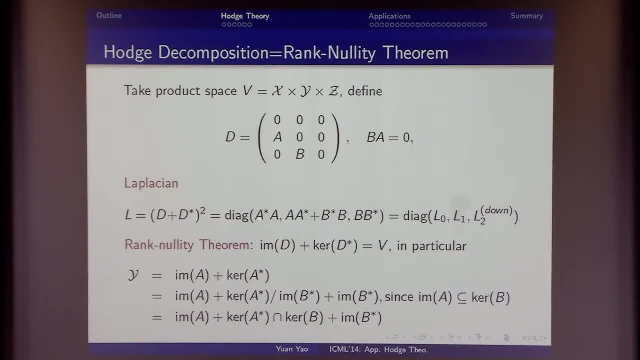 then you get this diagonal matrix. This diagonal matrix, the first part, the first element will be a operator only acting on X, the self action, And the second part is a operator acting on Y and the third part will be on Z And if you are careful enough, 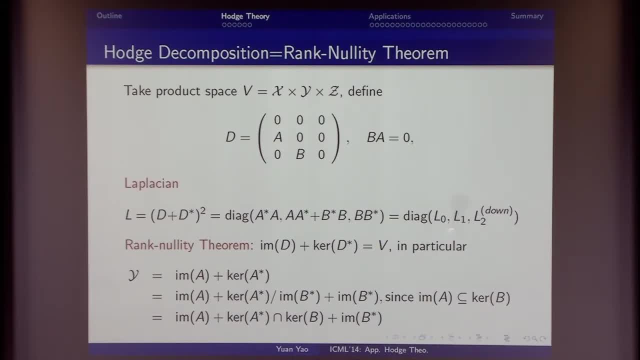 you can see when, later, when we develop one dimensional Hodge Laplacian, this sometimes called a graph Laplacian, This one sometimes called a one dimensional Hodge Laplacian, and this one can be used two dimensional by the lower part or down part of Hodge Laplacian. 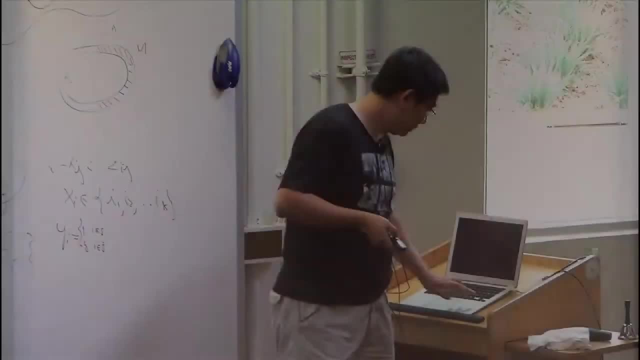 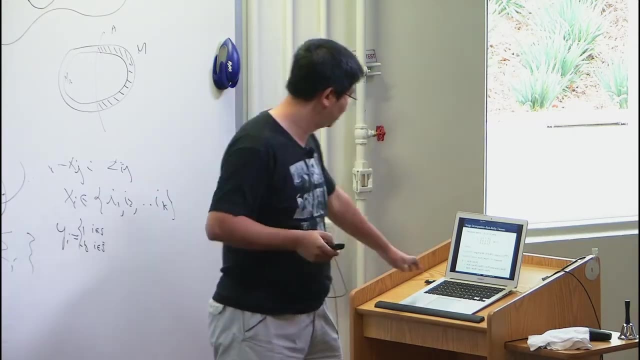 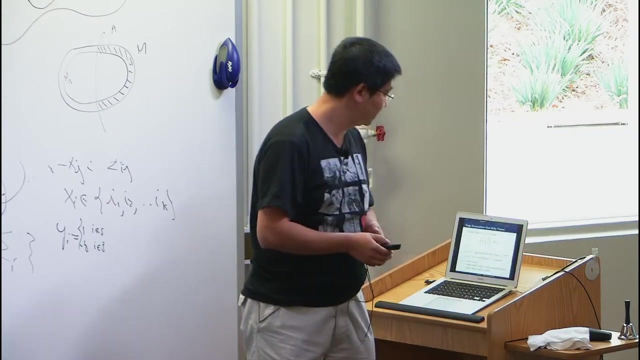 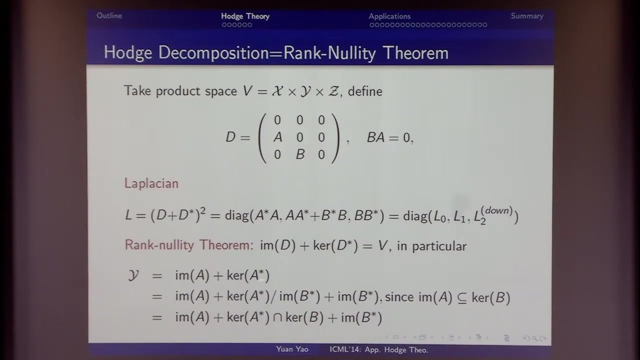 But this you can't forget, this kind of oh sorry, You can ignore the OK, Ignore this part for the moment. And these three lines just proved the Hodge decomposition using rank nullity theorem. Consider this matrix: the image of this matrix plus the kernel of its joint must equals to the whole space V. 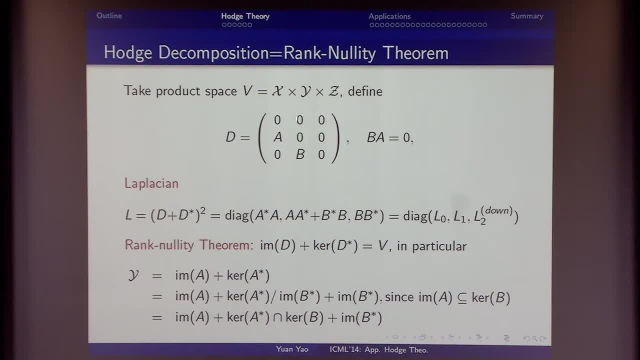 Then if we restrict everything onto the middle Y, what will happen? So in the middle Y the image of D implied by the image of A. So you take image of A here and a kernel of D transpose or D star, This one. 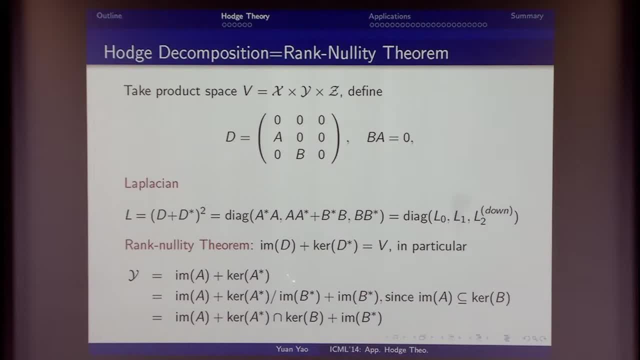 appeared here, will be kernel of A star. And this kernel of A star, because we know AB, this composition must equal to zero. So image of A must lies in the kernel of B. Then another direction: kernel of A star must include kernel image of B star. 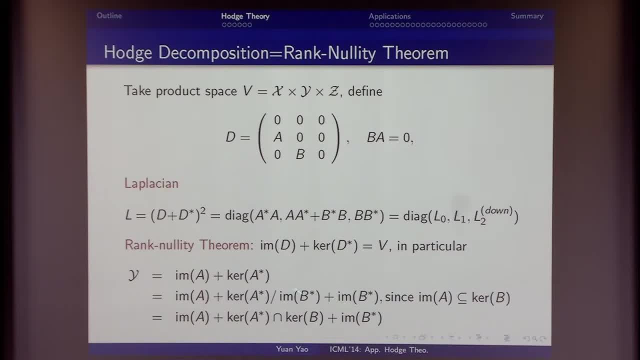 So if you plug in this term, decompose this kernel A star further into two orthogonal, orthogonal subspace. why is the image B star? Another is complement, orthogonal complement. Then in the middle you can replace this condition by the kernel of B star. 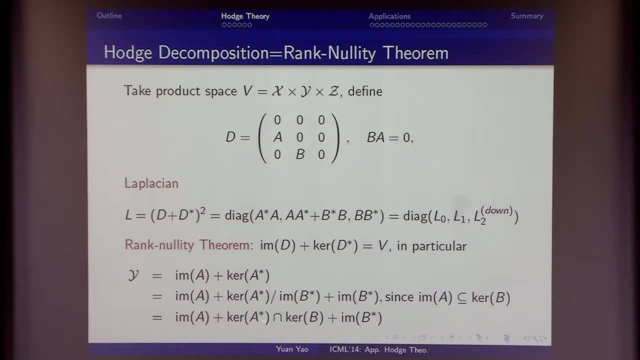 Basically the intersection of kernel A, star and a kernel B. This one gave this quotient space, So somehow from here you can see the previous slide, because this kernel must equal to the abstract Laplacian. And so in the middle, this Laplacian kernel. 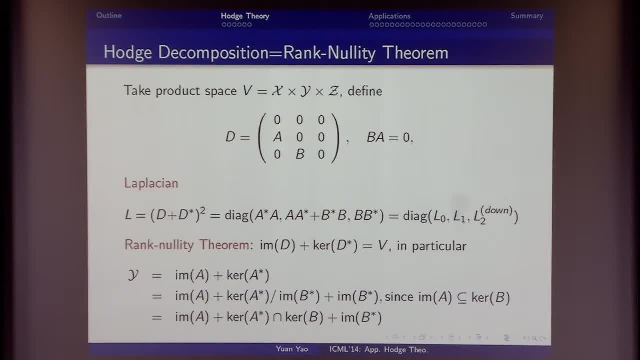 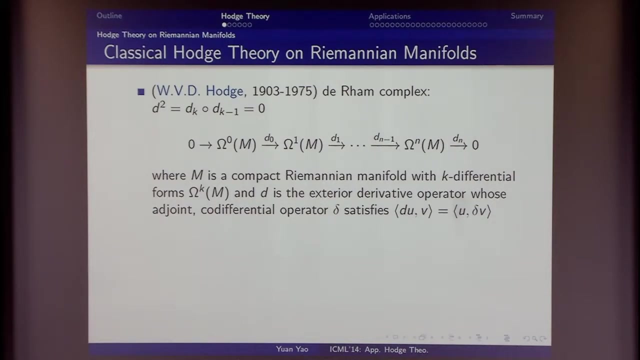 so you can put it here. So this is the rank nullity theorem derivation for the Hodge decomposition. So if you are curious, what's the linear algebra element behind that? So you, basically, you can follow this simple scheme. And now this simple linear algebra can carry various kind of structure in terms. 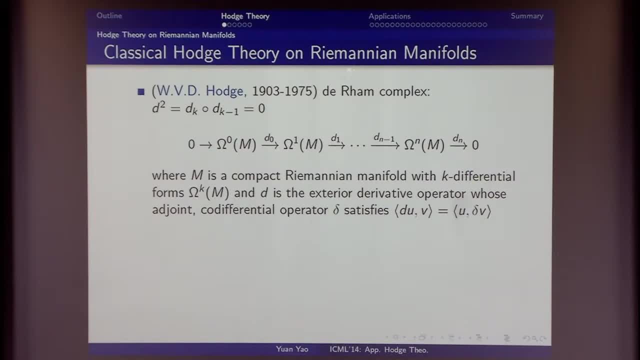 of different settings. The first version of Hodge theory coming from Riemann manifold, If you study the Dirac complex- basically you studied the chain map- becomes those X and Y and Z, Those in the product space, becomes the K differential forms on the manifold. 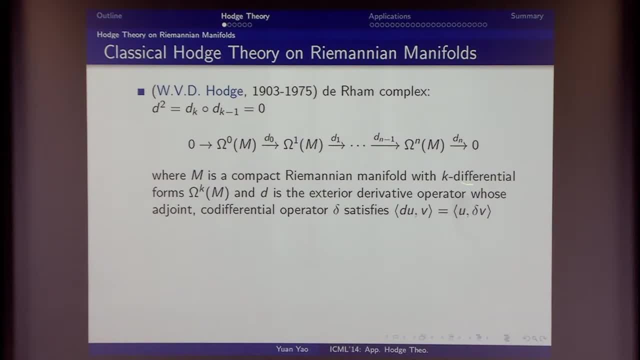 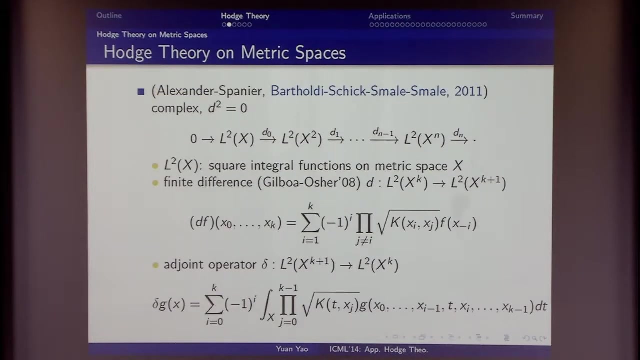 And the operator A and B, those operator becomes the exterior derivative operator And then you can define this kind of complex We call the Dirac complex and the Hodge decomposition naturally follows what we described before And another version is very recent work by Steve Smale and his collaborators. 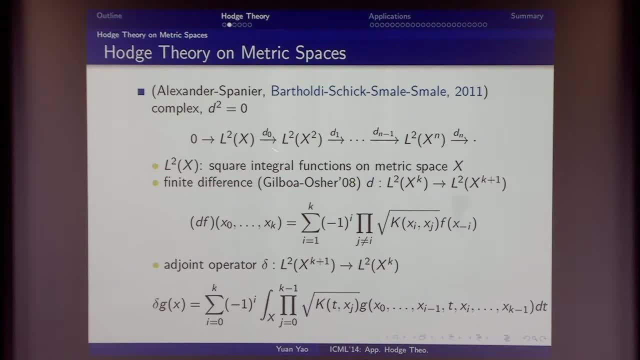 So they started the metric space and Hodge decomposition structure. Now the differential form becomes the square integral functions on metric space X And you can put finite difference operator, which are often used in numerical analysis and data analysis, And from low order to high order. defined in this way, 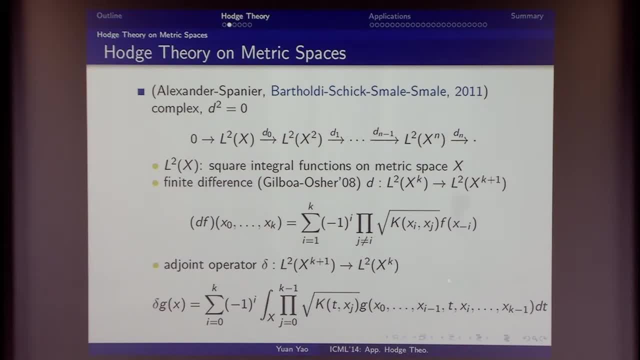 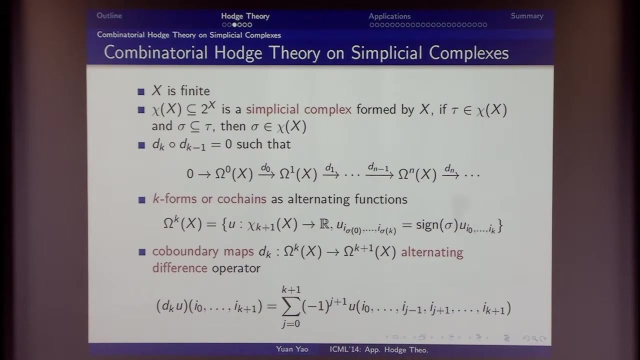 And you can define a joint operator- Basically they are the integral operator- and follow this direction. Then you can also find the D square must equals to zeros And the Hodge decomposition the algebra naturally carries here. So the third version is what I'm going to use in various kind of application. 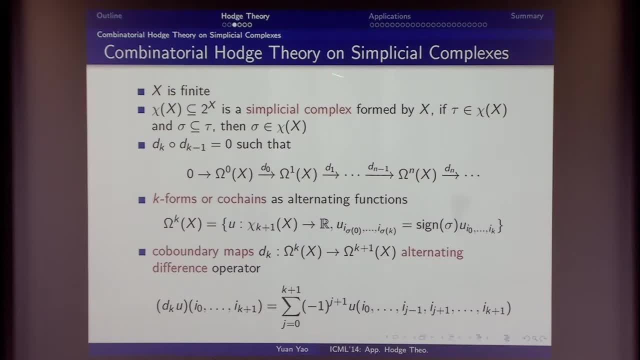 Below is finite version of combinatorial Hodge version. Basically we study a set, finite set X And we build up a simplicial complex, abstract simplicial complex- from X. That means we take a subset collection from X. 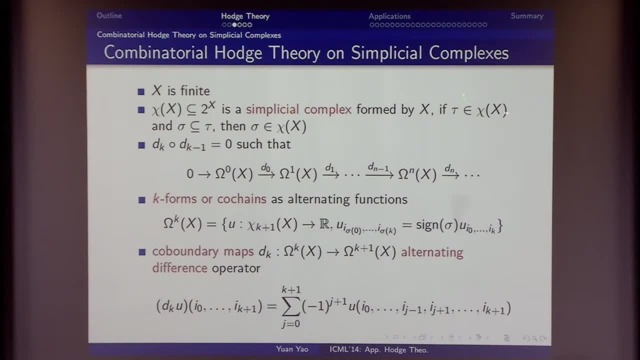 And if any set tau lies in the collection, then all its subset must be also included in the collection. We call this property as a closeness under the inclusion or deletion And when this satisfied we form a simplicial complex. Then you can define the K-forms as alternating functions satisfying. 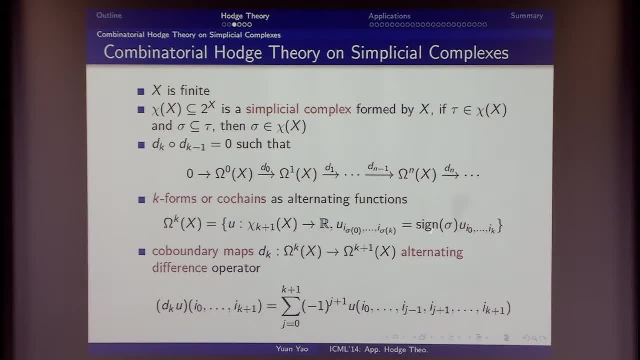 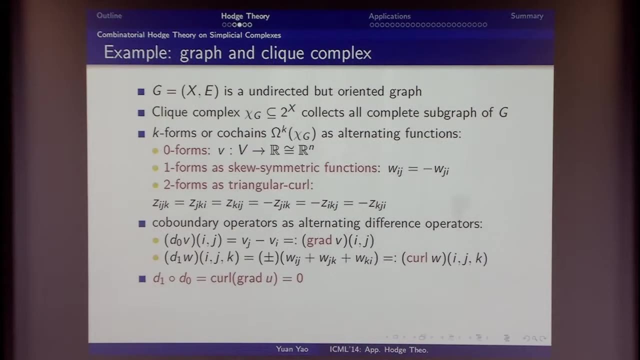 taking any permutation on the index set, you get a sign depending on the oddity of the permutation, Then it satisfies this kind of symmetry condition And the co-boundary map still is the kind of alternating difference operator. Similarly you can define a joint. 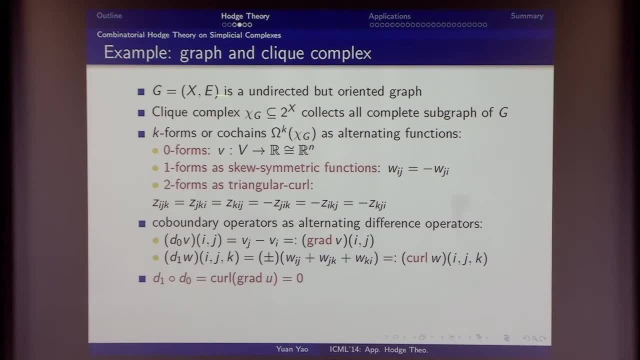 And now, if we take one particular example, consider a graph. We have an undirected graph but you can put orientation on the simplex, on the edge, And you can blow up the graph into a clique complex saying you collect all the complete subgraph from G. 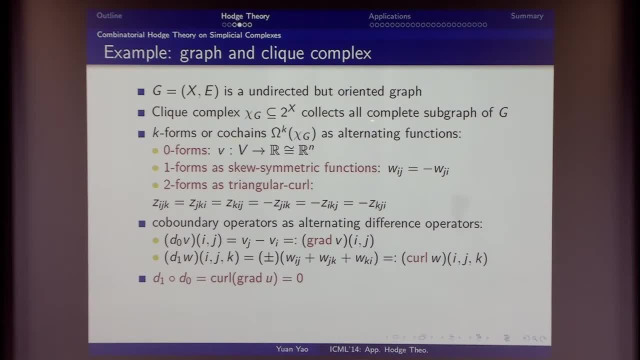 Then you form a collection. This collection satisfies the closeness and deletion. the property then becomes a simplicial complex. Then with K-forms you can define something like that for zero form. Basically it's a function on the vertex set. 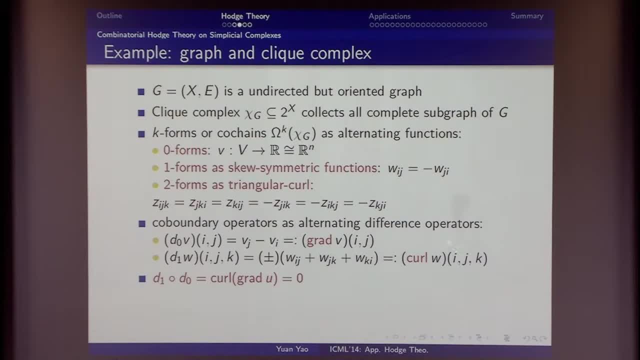 For one form it's a skew-symmetric function defined on pairwise vertex, on the oriented edges, And two forms basically are triangular curl. It satisfies this kind of alternating symmetry. Then you define the function on the oriented triangles, So co-boundary operator, basically just difference operators. 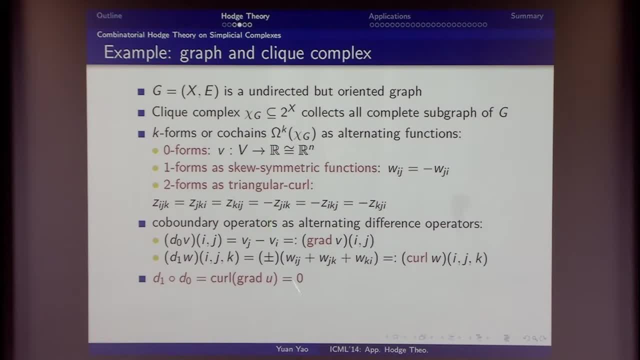 And if you take a map from zero form to one form, that forms the finite difference operator on the graph. If you take from one form to two forms, then basically you take a triangular trace along the orientation of the triangle, Basically depending on the orientation. 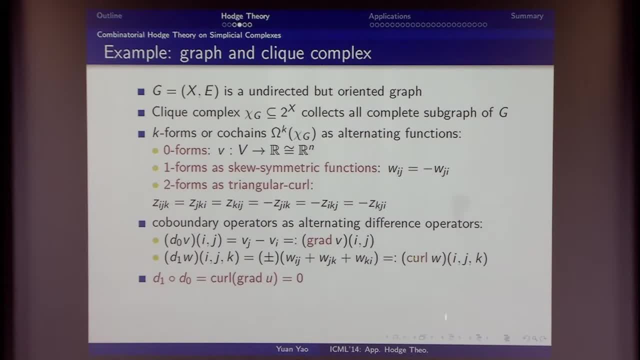 you can put a plus or minus sign there. We call this kind of operator as curl And similarly if you define the inner product, natural Euclidean inner product or anything associated with this form, you can make a joint operator of them. And the most important property is curl of gradient field must equal to zero. 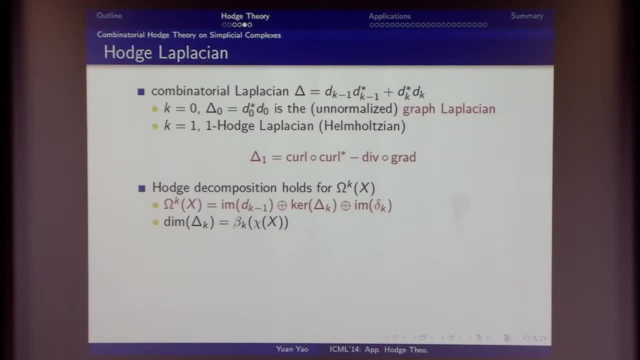 So this you can understand it from very basic multivariate calculus And one-dimensional combinatorial Laplacian will be defined in the abstract way like this: And, in particular, if K equal to zero, that becomes the graph Laplacian, But if you get a K equal to one, the one-dimensional Hodge Laplacian. 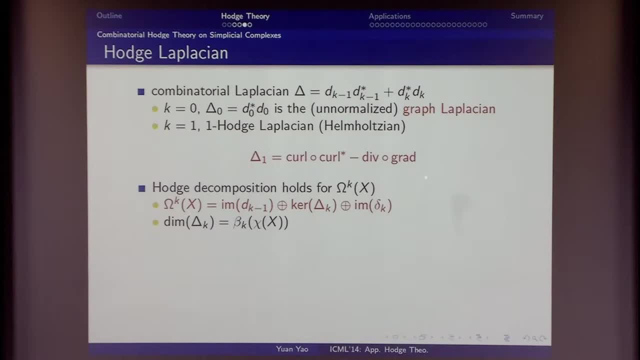 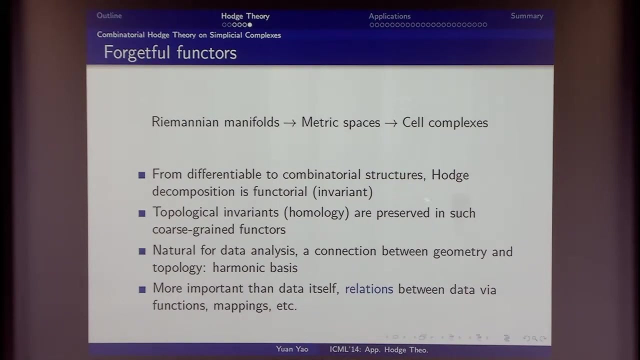 will be very useful in the later development, like game theory, decomposition and ranking decomposition, And these are things the same as before the linear algebra part. The useful things. why this kind of structure repeatedly used from manifold to modern data analysis? because remaining manifold and metric space and cell complex. 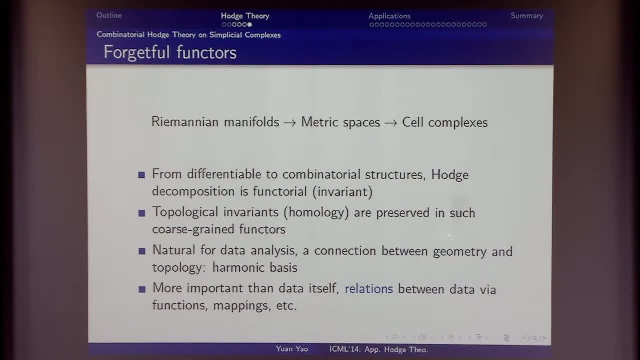 whenever you forget some structure like metric space, metric structure, differentiability structure, but everything invariant preserved with this kind of linear algebra And that reflects some topological invariants, like homology, reflected in the dimension of kernel of Laplacian. So we don't need those high sophisticated structure. 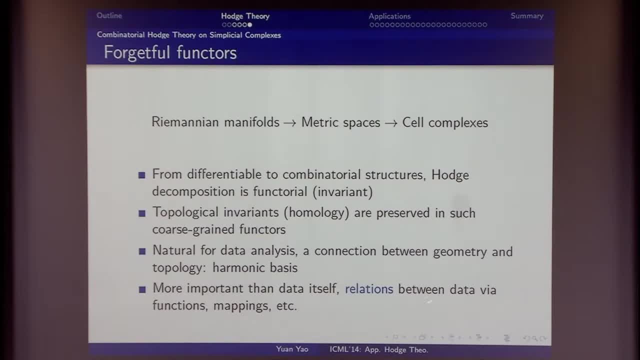 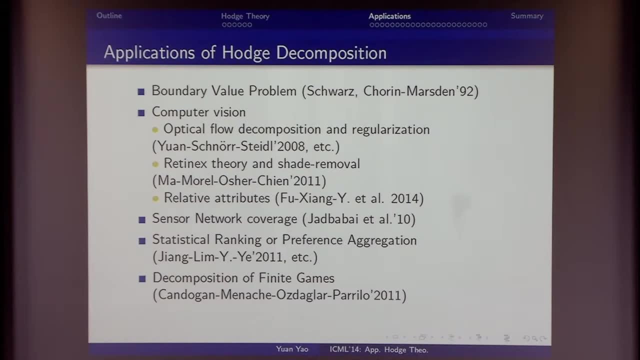 but with cell complex, very natural fitting for data analysis. So we expect this kind of property may make Hodge theory appear in various kind of applications. So the classical application for Hodge decomposition is boundary value problem in PDE And very recently there appears a lot of new application from computer vision. 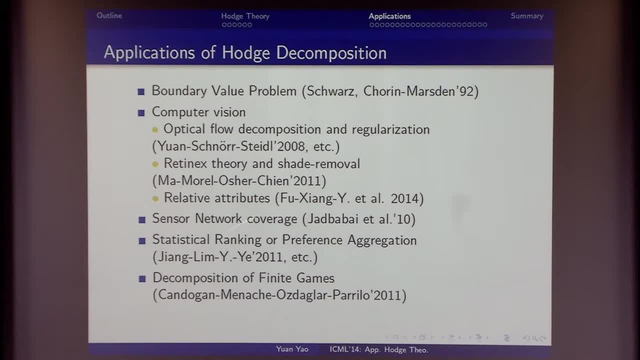 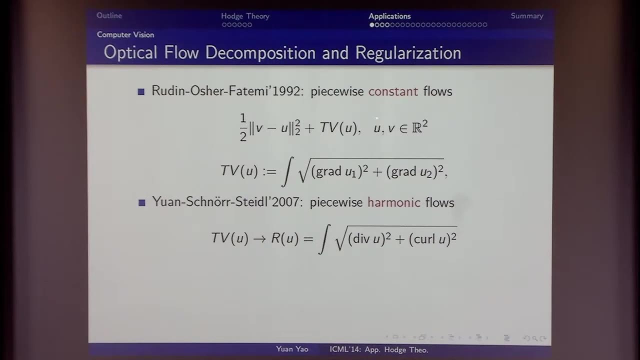 and to sensor network coverage and statistical ranking and finite game decomposition. So I will pick some of them to illustrate how the idea might be used in various different kind of setting. So the in computer vision very well known model called the Rudin-Oscher-Fatami model. 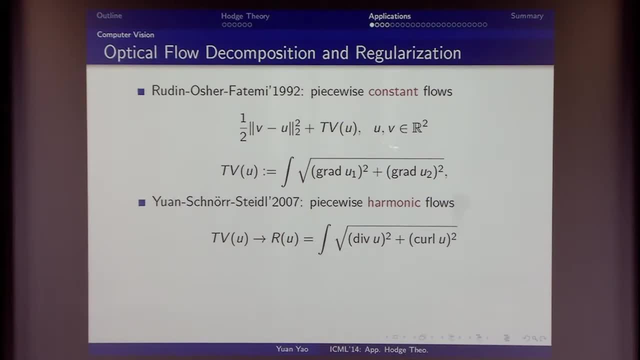 They study piecewise constant flow, approximation, given a kind of given an image on the plane, for example on two dimensional plane, And the piecewise constant flow basically represented by the total variation and regularization term. This one, basically a L1 norm, for if you take this one, is a group as a complex. 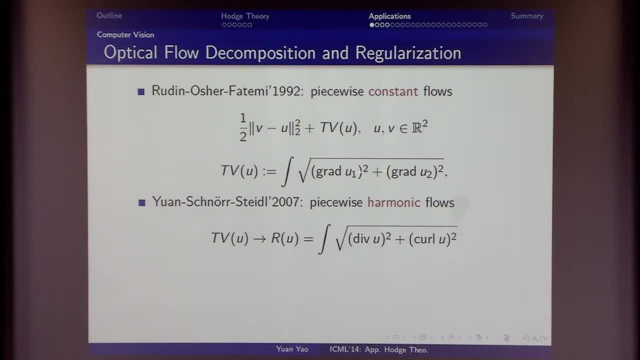 member in the plane. In other language, like statistics, they can call it a group lasso. So this one favors the piecewise constant flow. But why we have to use a total variation? as to use piecewise constant flow to approximate our original image. the intuition is a piecewise constant flow may help you to preserve. 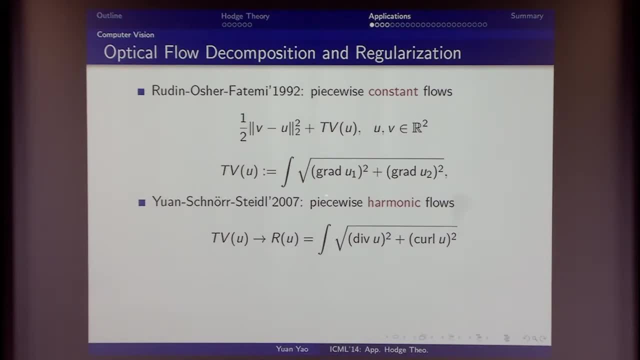 the edge in the image. However, if the flow, if the original image coming from videos or image sequences, they are often some objects in the videos and the object may undergo certain movement. So in that case piecewise constant flow may not be a good regularization to. 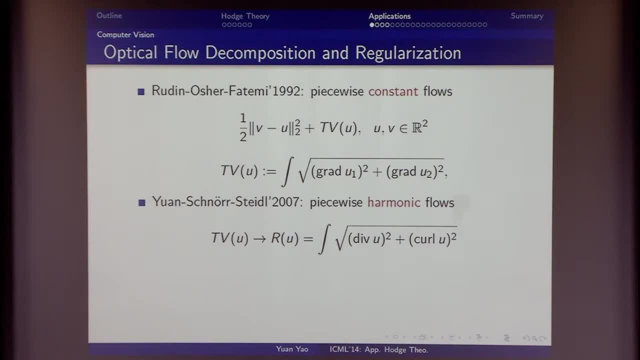 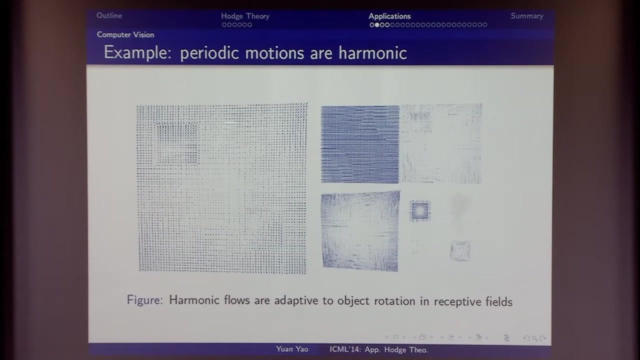 preserve the object, the edges associated with objects. So recently people suggest use a piecewise harmonic flow to approximate our original one, And this one becomes useful to study the optical flow problem in the video processing. So here it's not quite clear to you, but basically it says that there are 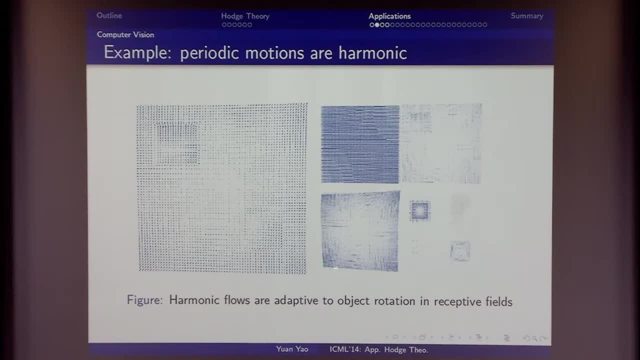 some object in the receptive field and that the object undergoes some rotation movement. And if you use a piecewise constant flow then you totally broke the object boundary. But if you use a harmonic, piecewise harmonic flow, then that very adaptive to the objects. 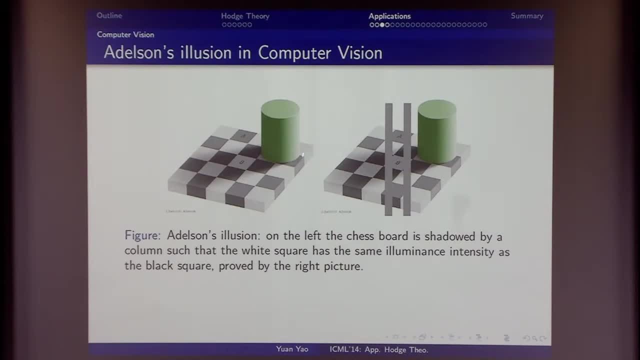 So illustrate this kind of application, Another application from computer vision, So this example called Ellison's illusion. for example, if you put a pillow, a column on the chessboard and the column leave you some shade on the board. So basically there are two colors: white and black. 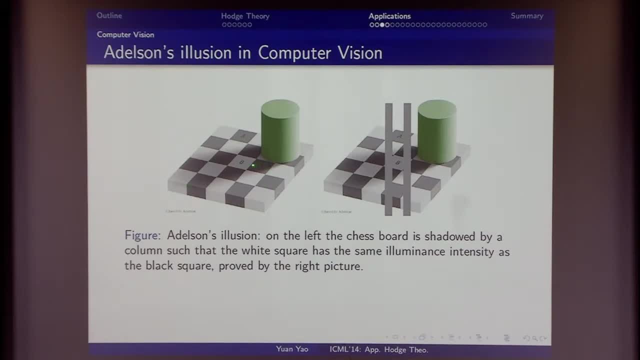 But under the shading the absolute intensity inside of the shade will make the white white part looks like the black part outside of the shade. So this is the illustrate. So this black part has absolute intensity level at the same level as this white part inside the shade. 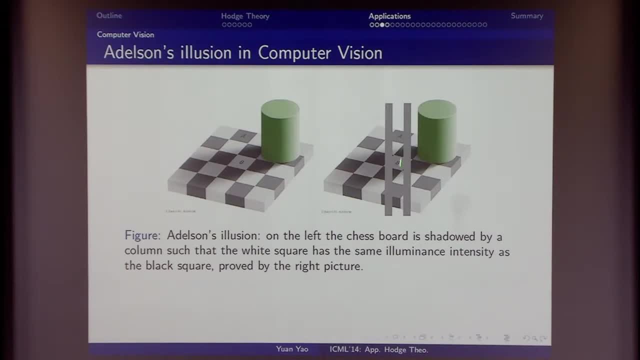 But although this one happened to be the same of intensity level for you, you never get confused. This is a white, This is not white. This should be black, This is white. You never get confused with these two. How this happened in for human eyes, and people suggest that because human eyes. 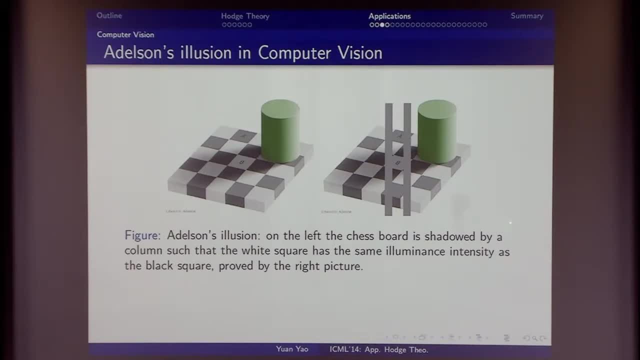 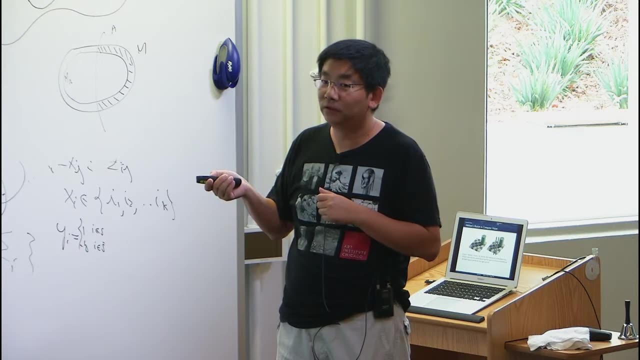 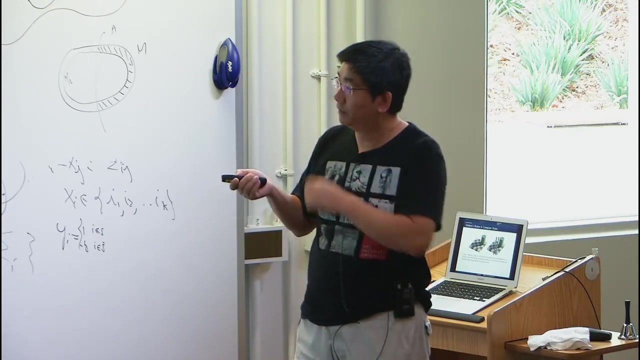 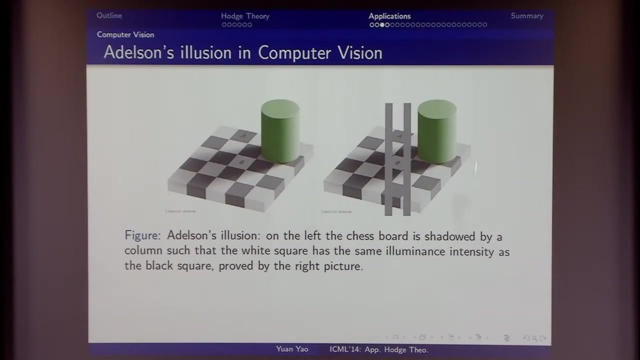 only use the sorry quick question. So you mentioned the cell complex earlier. So are we striking as arbitrary cell complexes or as once embedded in some dimensional abstract? abstract, Yeah, it can be abstract and can be embedded, Yeah, And and for this version, and people suggest to use a pairwise contrast to to reconstruct. 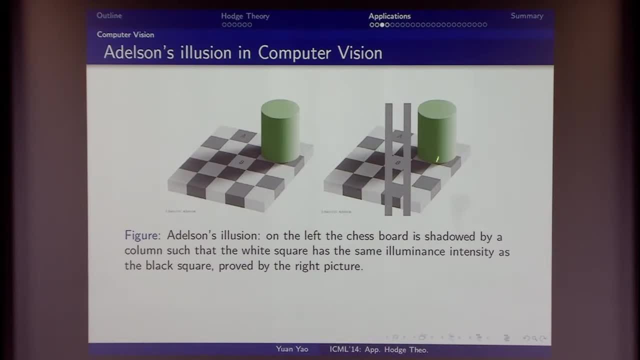 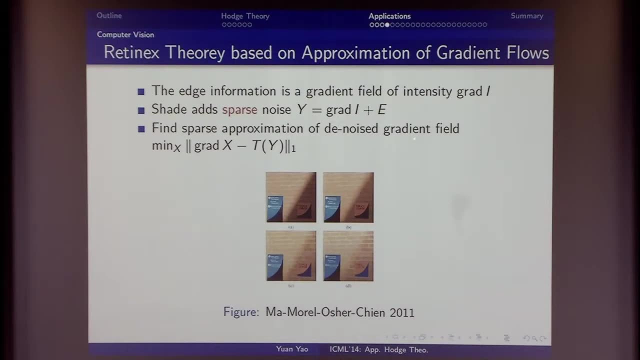 the image. That means that we look at the vector field derived from the gradient of the original image and then use a truncated version to remove the noise, then reconstruct using some sparse reconstruction. So this kind of approach suggests by Osher that sometimes it can be related to the Hodge decomposition. 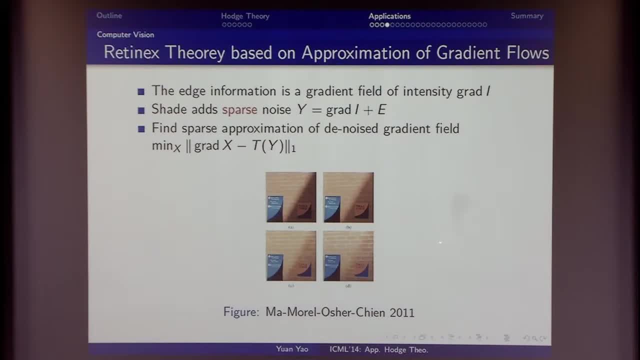 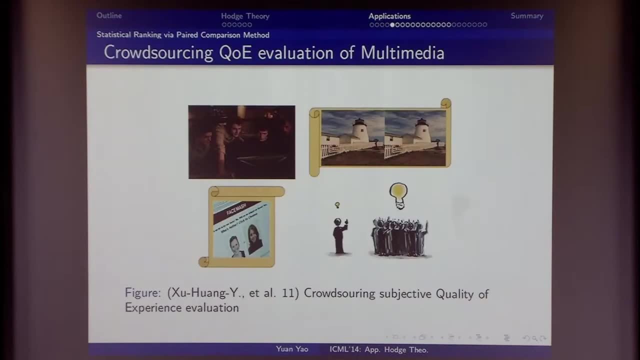 but it may not be out to the version Hodge decomposition So if you are curious, maybe you can sing from this kind of direction. So this second example is from computer vision. The third example actually is from multimedia society, a small society within the computer vision. 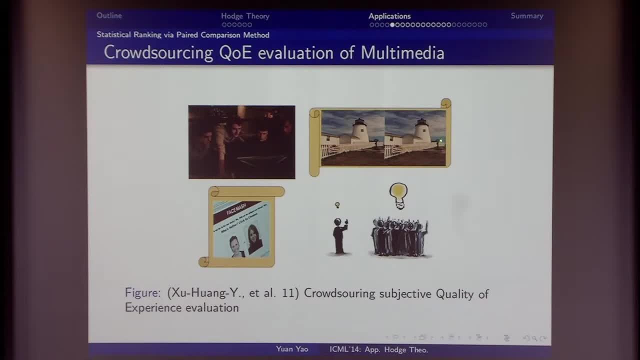 And people want to wonder. You have lots of videos on the YouTube, for example, or Facebook. You have lots of pictures and those multimedia content may be the same. But company need want to know if we adopt certain data compression technology and how the video contact. 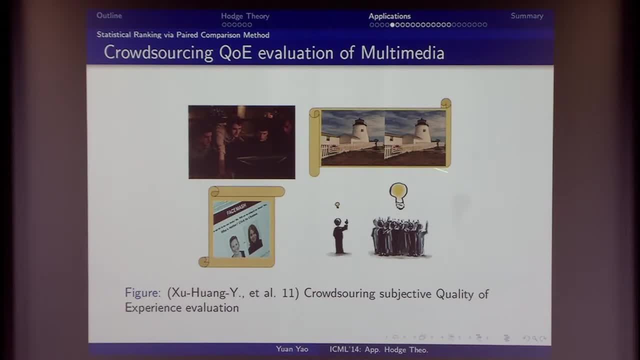 Content looks good or bad for the reviewers, for the crowd on the Internet. So basically they adopt a crowd sourcing quality of experience experiment, Try to evaluate how the technology looks good or bad. So this is kind of another resource for pairwise comparison with a crowd sourcing. 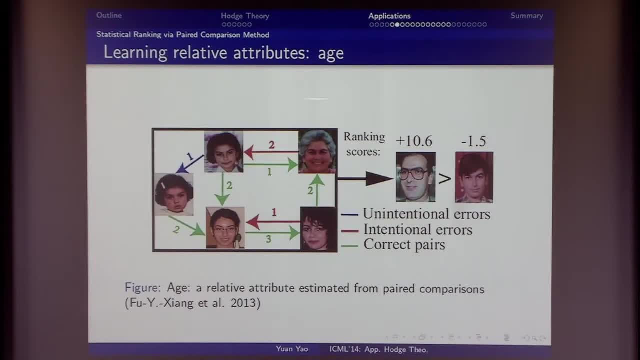 experiment emerged recently and this particular example from computer vision called the learning relative attribute. Given a pair of a, given a face from the Internet and you ask a question- How old this people looks like- It's very difficult for you to give any answer. 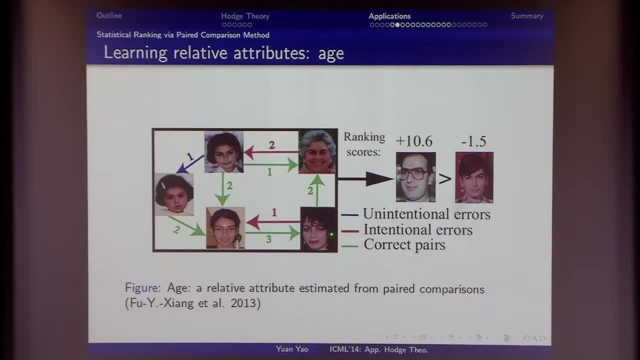 How old. But if you are given a pair of images then relatively you are easy to tell which one looks older, which one looks younger. So this kind of application we use a relative, We call the relative attribute, and age is only one example. 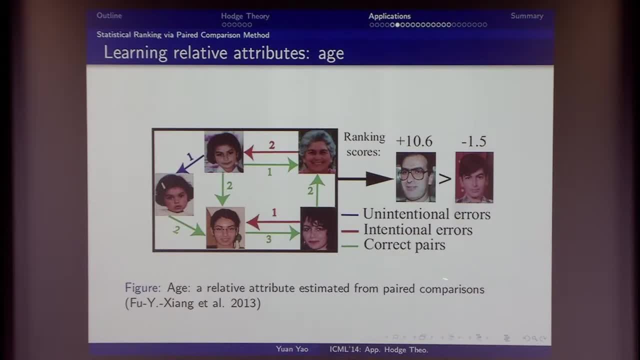 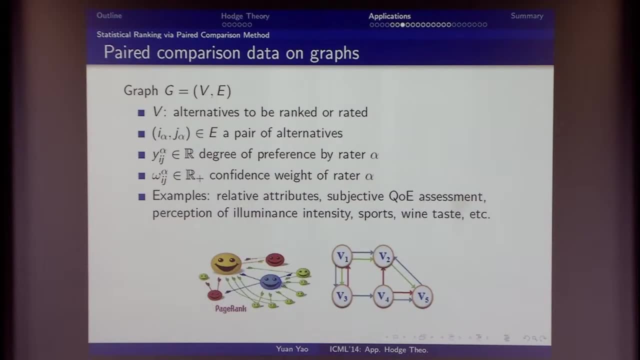 And the people adopt a pairwise comparisons and from to collect the data using crowd sourcing platform on the Internet. So all these kind of data can give you this kind of abstract problem. You are given a graph with the vertex set those alternative to be ranked or compared. 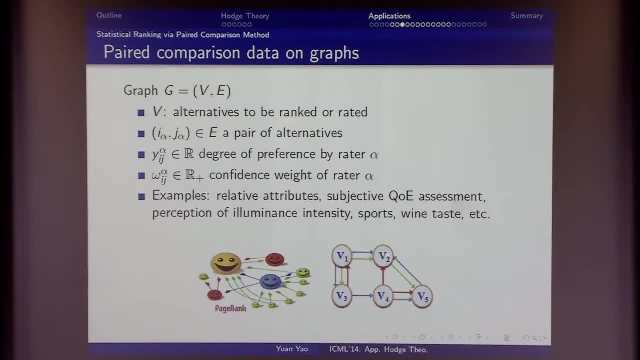 and the edge set consists of a large number of pairwise comparisons and people. different people may vote different colors and hear some different color, And if you trace back to the classical page rank, that's the one particular version for this, for this kind of data. 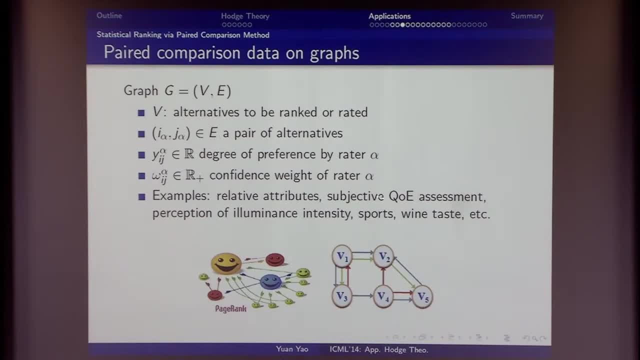 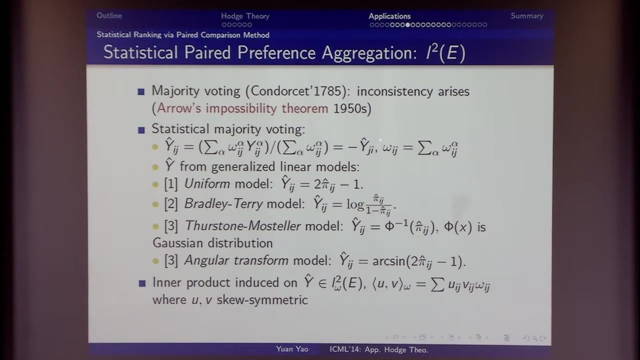 But more data nowadays rise from multimedia and the computer vision and wine taste, psychology study And this kind of data, how to aggregate into a consistent global preference order or global ranking? This is very classical problem If you can trace back to the social choice theory. 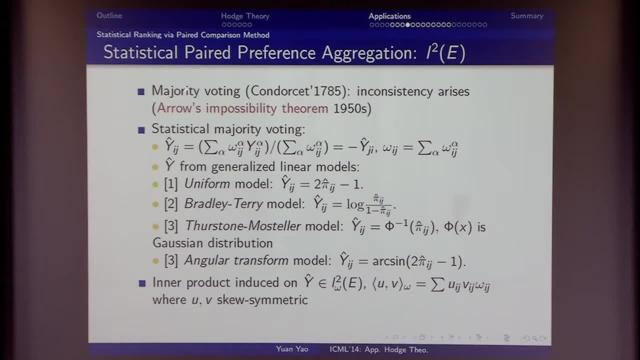 So it start from the 18th century and people know that at that time majority voting may arise some inconsistency and especially arrows impossibility serum says that if you follow the majority voting then all the kind of ranking chaos may happen. otherwise, except that you take 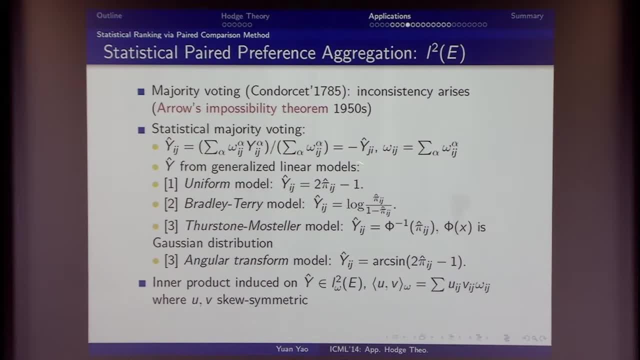 a monopoly structure in the fine social society rule. But where is kind of interpretation for arrows, impossibility serum? But in practice people still use a statistical majority voting And the question is how much you can gain from impossibility you, how possible you can do that with that. 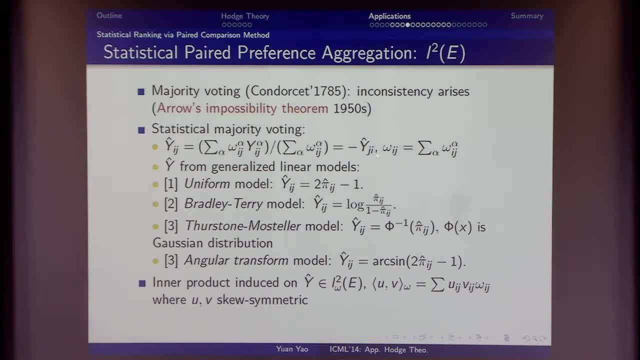 And so here is a from statistical society. people can aggregate the pairwise comparison using virus kind of models, depending whether the data is a preference degree or binary choice. You can choose various kind of models, and all these model give you a kind of abstract data. You have a pairwise comparison data which are lies on the edge space and which are square, integral. 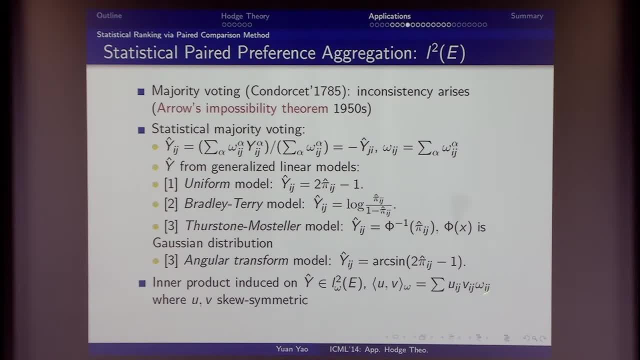 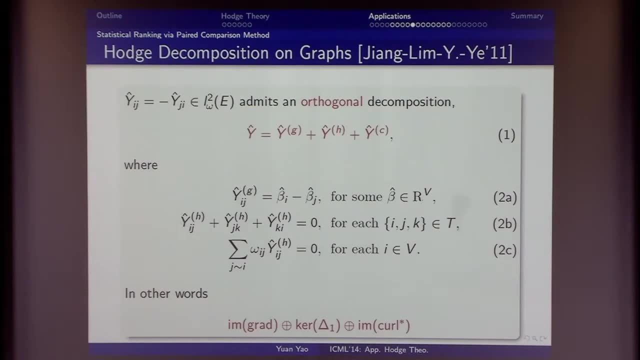 or in the certain sense and with certain inner product defined by the confidence level. So if you have such kind of data, the Hodge decomposition basically tells you this one. any kind of data coming from the stochastic majority voting admits such a orthogonal decomposition and the first component, which is a gradient, 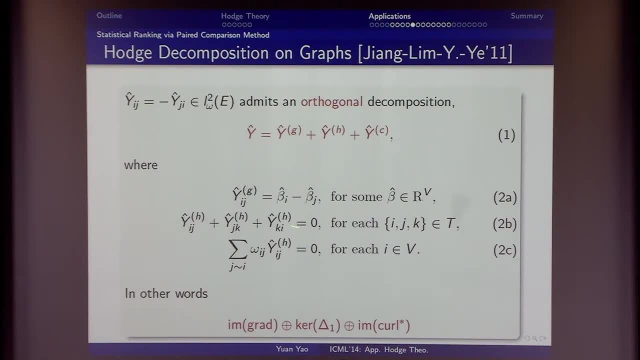 of certain scaling function on the vertex side. Second, the component actually satisfy this triangular curl equal to zero and simultaneously it has to satisfy the divergence with equals to zero. We call the curl free and divergence free And these two condition uniquely decide the orthogonal projection component here. 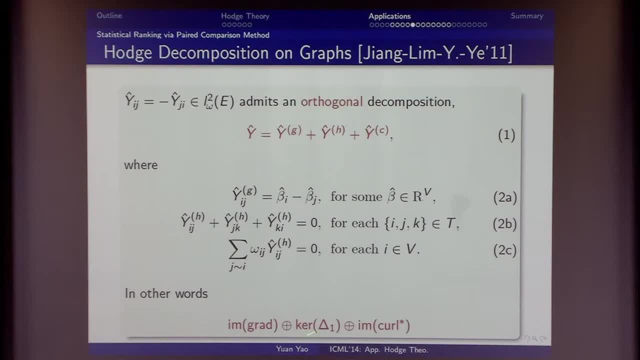 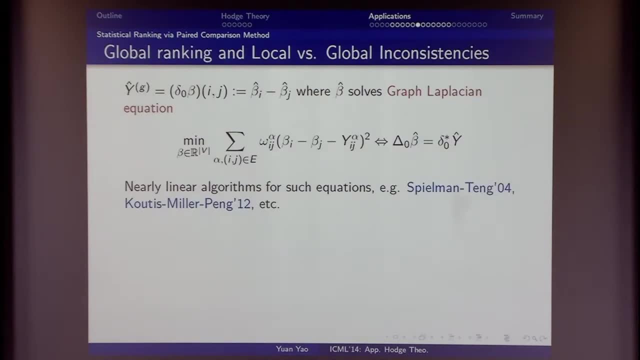 And in other words, if you put that into a Hodge decomposition means such kind of data always has this kind of Hodge decomposition. The question is, how can we find these? each of the component, The first component, actually basically solve the graph lesson equation. 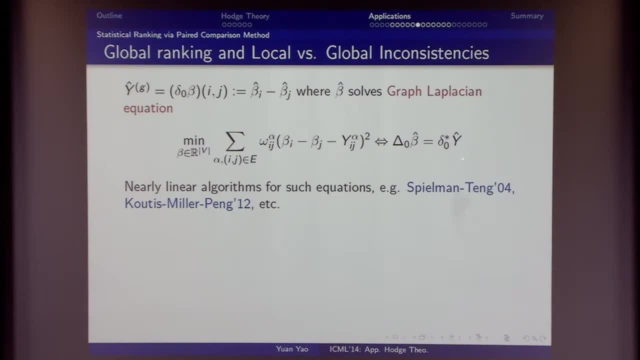 And satisfy you this one. And the good news is recently people knows that for those graph Laplacian equation We have nearly linear algorithm but means they are kind of suggestions from a society like a Spearman and Tom and Gary Miller's group. They are try to make this kind of algorithm more practical in the practice. 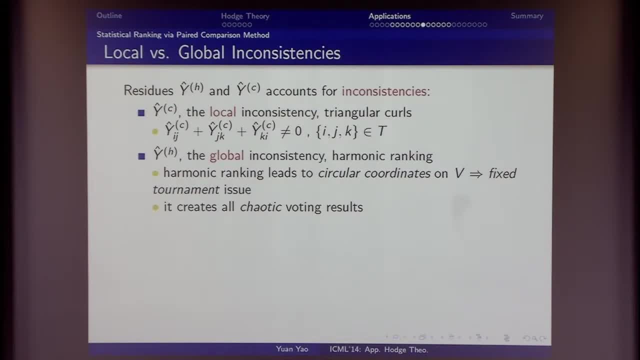 But the part of part coming from the second part. So how to compute the harmonic and the curl part. So this is a kind of difficult. So what's the meaning of these two part for the third part, curl part? actually it comes for local inconsistency. I call because on every triangle the total curl should, should not vanish. 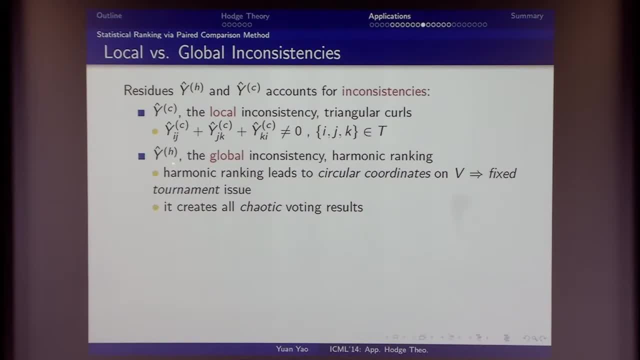 But the middle part is a kind of tricky because it satisfy both triangular Curl free and the divergence free. basically it gives you a circular ranking We call the harmonic ranking, and this kind of circular ranking that generically will pass all the vertex set. So give you a total round order and those vertex set. 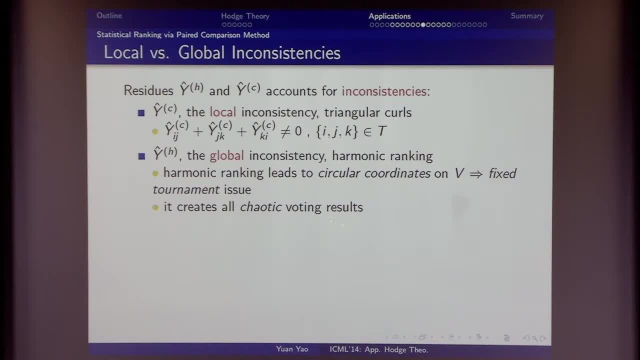 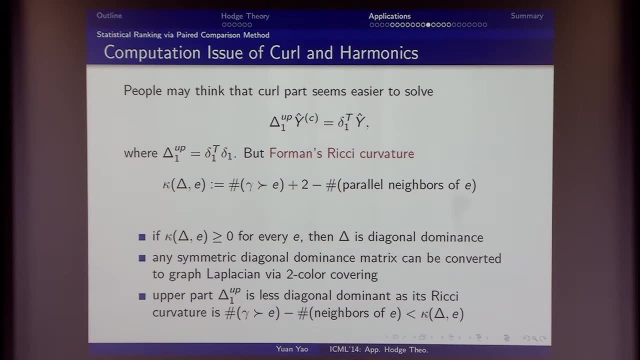 So this one creates all the chaotic voting result once you have any component like this, So this probably the hardest pass in ranking. But the question is how to compute them, And people may think that the curl path seems easier to solve because every Hodge Laplacian has the upper one and lower one. 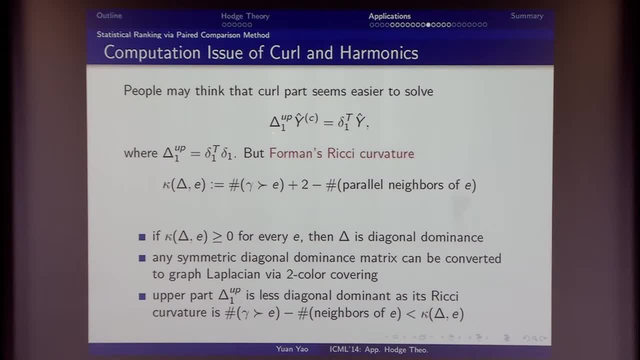 Talked by Liheng and Cheyenne, And you can solve this upper one solely when you get a projection on the curl part. But the question is the upper part in terms of the pulse, in terms of Laplacian kind of progress. 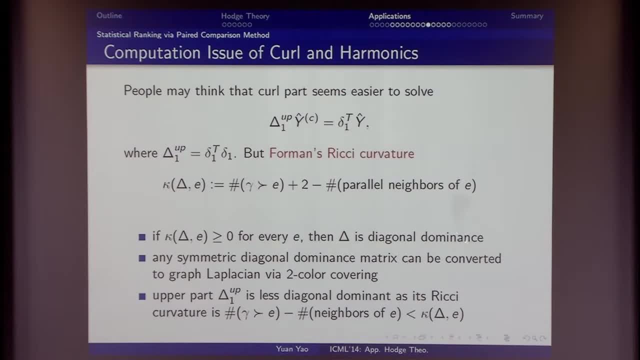 The third, the this curl part equation, is not that easy, because this one is far from, far away from the being diagonal dominant. In fact, if you look at the formants of Risi curvature defined for the Hodge Laplacian, The form that means if this quantity is non-negative for every edge, then this one Laplacian must be diagonal dominance. 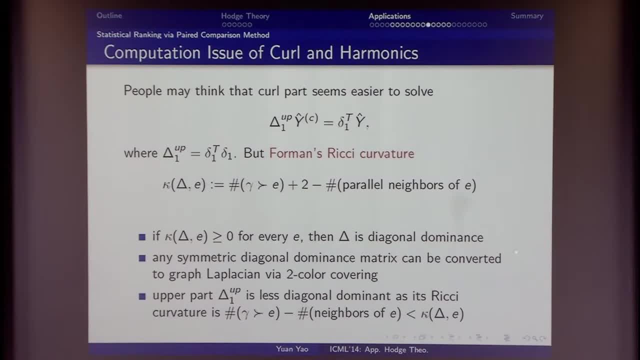 So this is a kind of equivalent condition for the one Laplacian to be diagonal dominance. So we know, if the Laplacian is diagonal dominance, this although it's one Laplacian, we can always convert this Laplacian to be some graph Laplacian using some two color covering. 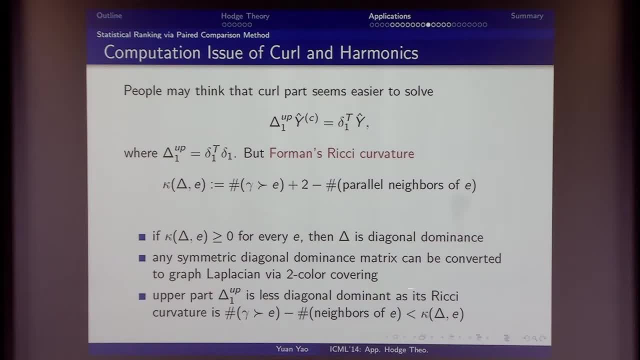 And then you can follow the previous technique for graph Laplacian equation, solve it efficiently. So we can find the harmonic ranking much more easily in this case. But in general, if it is not diagonal dominance, things might be harder. But the question why the upper part might be harder to solve than the whole one Laplacian. 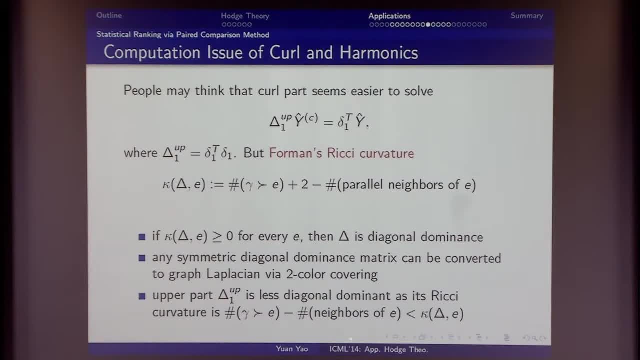 Because if you look at upper part, it's Risi curvature is always smaller than the total, the whole one Laplacian part. That means it tends to be more negative than the diagonal dominance one. So this one is: if you pursue the diagonal dominance kind of technique, perhaps this upper part is much harder to solve. 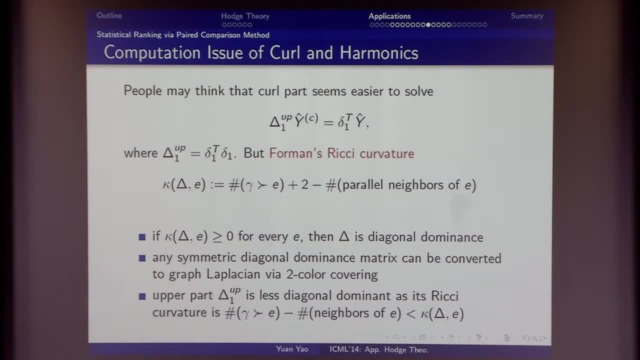 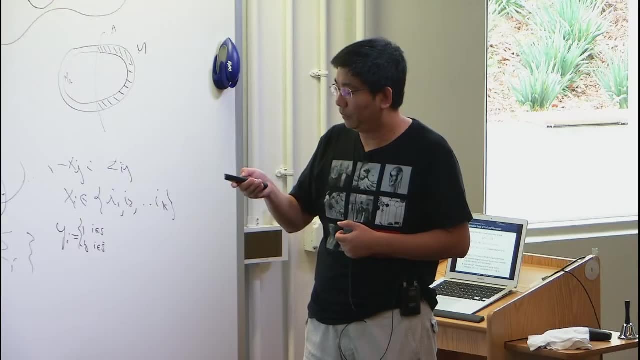 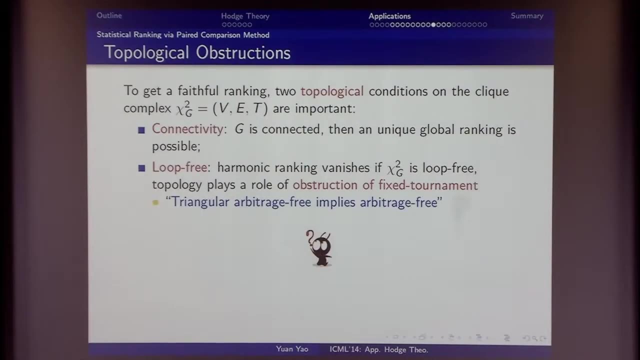 So I'm not sure whether this is a good reason to persuade you to move to harmonic ranking computation rather than the curl computation, But there are lots of things inside this kind of question, So this is a good reason to consider. And the topological obstructions in Hodge decomposition, because it relies on the connectivity and whether there is a BT1 or loop in the clique complex. 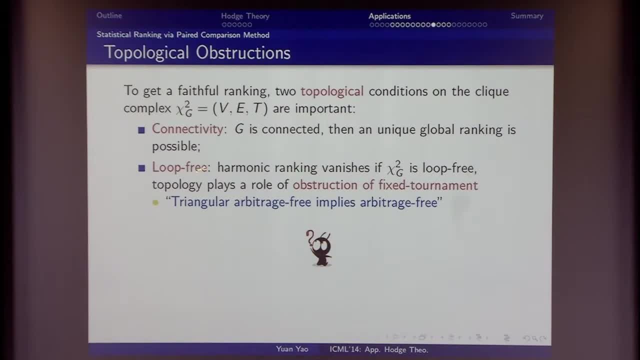 So if the clique complex created from the graph is connected, then we can get a global ranking up to a translation constant And if it is further loop free, then every harmonic. you don't have any non-trivial harmonic ranking. Then you won't have this kind of circular coordinate which creates all the voting chaos. 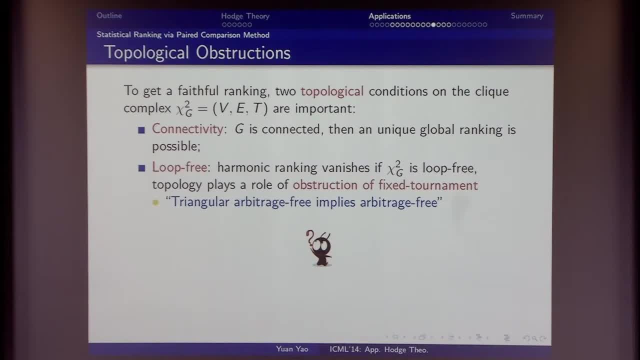 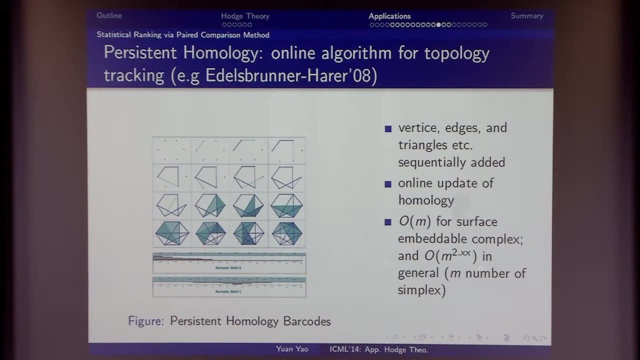 So how to track the topology change. So basically we have, using the persistent homology, we can have a polynomial algorithm up to number of cells, or simplex, And the simplex complex up to the power. two point- something It depends on future development- and basically you can use this kind of algorithm to do the 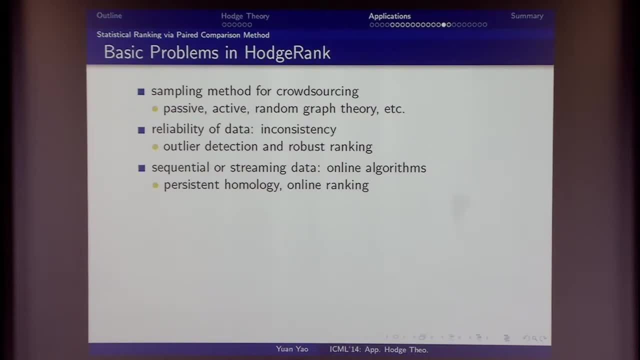 It gives an online algorithm for topology tracking if the simplex sequentially enters the stream And the virus kind of problem in Hodge rank when you try to apply it for cross-sourcing study. and I just listed some of them. First important thing is how to design. 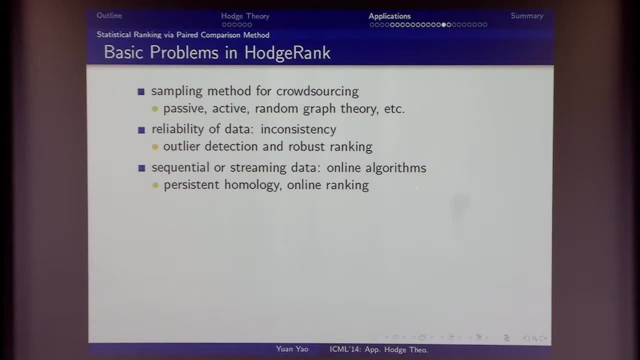 Sampling scheme, and so here you can use random graph theory to guide your study. And the second thing is how much reliability, how to deal with the reliability of data, And we can divide of outlier detection and robust ranking. And the third one is how to face the streaming data. 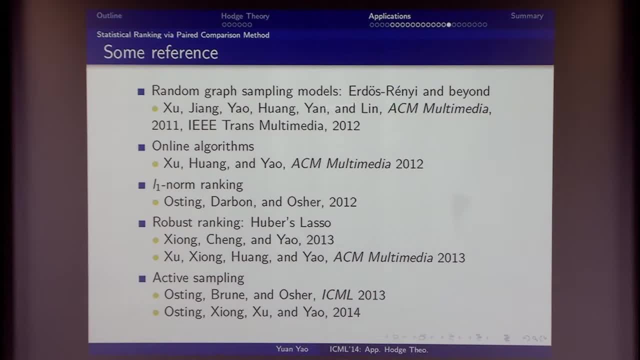 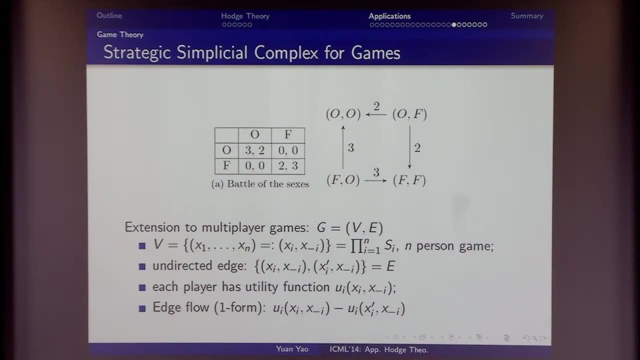 You need some online algorithm. I won't talk too much about these things And if you are interested, you can look at those reference which appeared in our collaboration And some people in Osho's team recently. So here I would like to give you another application. 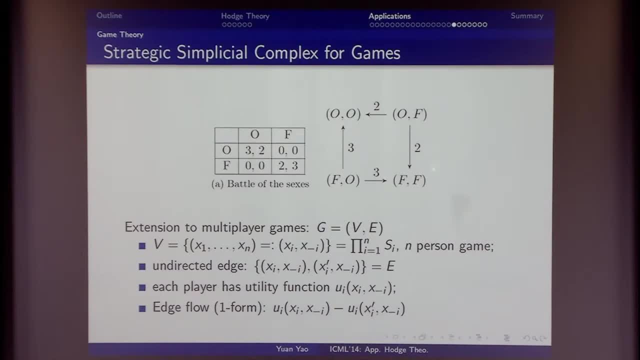 So this is one of my favorite example of Hodge decomposition application. So you can use Hodge decomposition to study finite games. In fact, every finite game can be decomposed into the Hodge structure And that corresponds to zero sum and potential game. 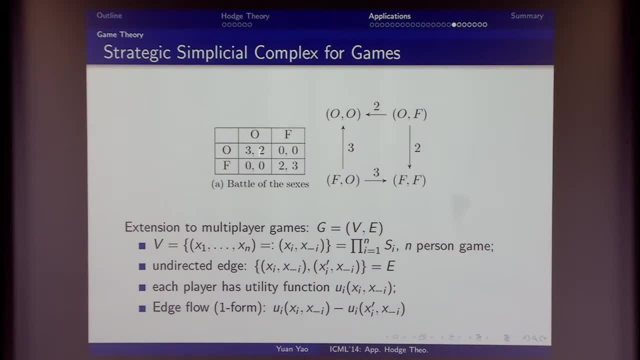 Very well studied topics in game theory. So if we look how to convert the data- game data- into the Hodge decomposition structure, Basically you can look at all the standard form for the normal form of the game. So for example, here is the battle of the sexes game. 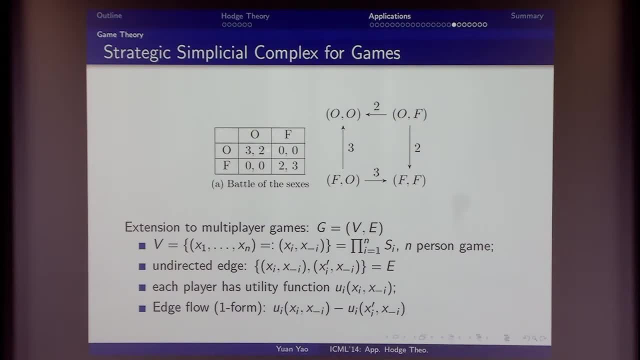 So you have two person- wife and husband- And each one has two option in the weekend to choose whether they go to see the opera or they go to see the football. And if the husband and the wife both go to the opera, then the wife will be more satisfied. 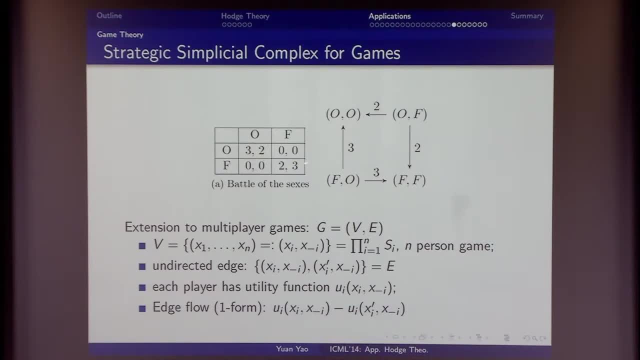 But the husband will be a little bit less satisfied. And on the opposite, if both go to see the football, the husband will be much happier than the wife. And the sad thing is, one go to see opera, another go to football, And depending on whether the husband like the opera or the wife likes the football, the number can varies. 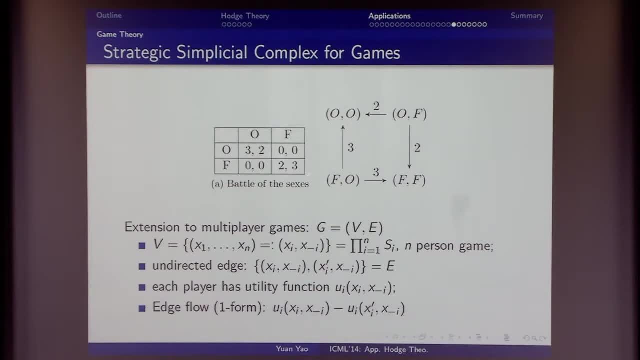 But you can put such matrix as the payout function for each of the player. So the question is: we need to make a graph representing this game. The graph basically consists all the vertex sets As each player, all the player, put their strategy as a vector, then put the vector profile, strategy profile, as a node. 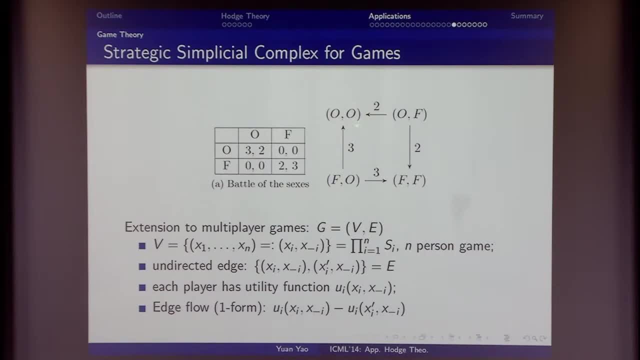 Then you make up a large graph. each node represent strategy profile And how to put edge between the nodes. So one choice suggested by Pablo Parello's group is: if only one player change their strategy, Then you use edge, add edge between them. 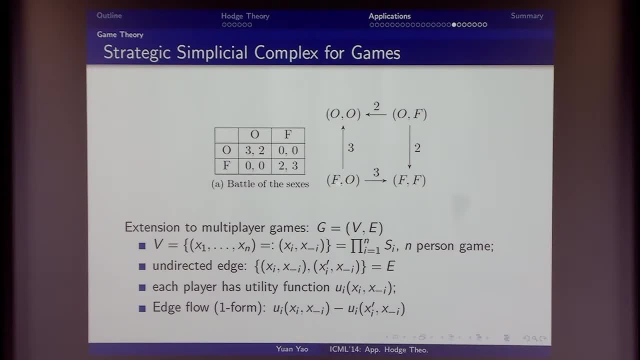 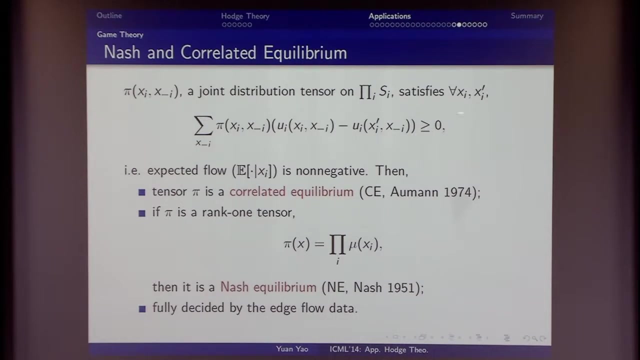 So that means two strategy profile are comparable, if only one user change strategy, Because in that particular case you can use that particular user utility as the edge flow. So that maps the data on the graph in this way. So If you take such a data, basically you find you can preserve the Nash and the correlated equilibrium. 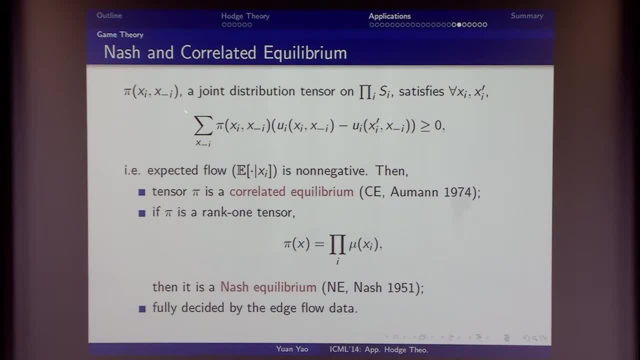 With respect to this kind of data- graph flow data- And suppose you have a joint distribution on the strategy profile space And which is basically tensor, Depend on how many players have You have a high order tensor And, if it is satisfied, this kind of linear inequality. 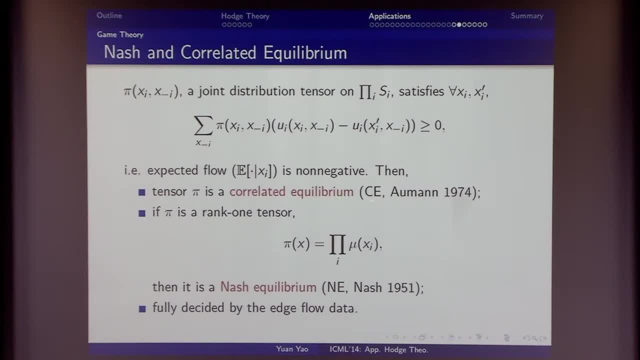 Then this tensor must be equilibrium. And in literature Allman called this one as correlated equilibrium. And if you take a rank one tensor, If this one is rank one means every player independently choose their strategy satisfying the same set of linear equation- Then that's called Nash equilibrium. 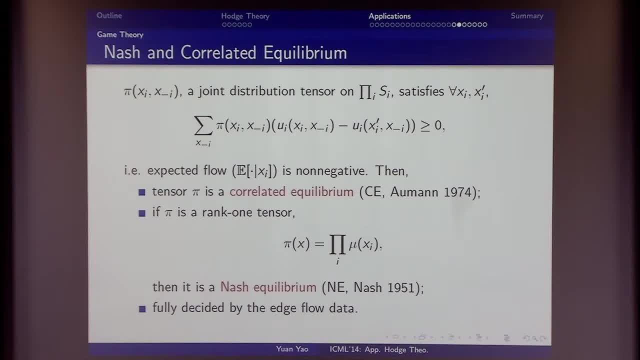 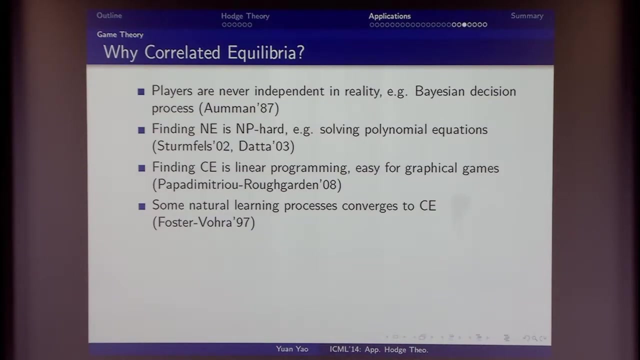 And both equilibrium actually can be fully decided by the edge flow data. When we map the game onto the graph in this way, We don't lose any information about the equilibrium problem, And the question is which equilibrium we should look at. So this is very complicated problem in game theory. 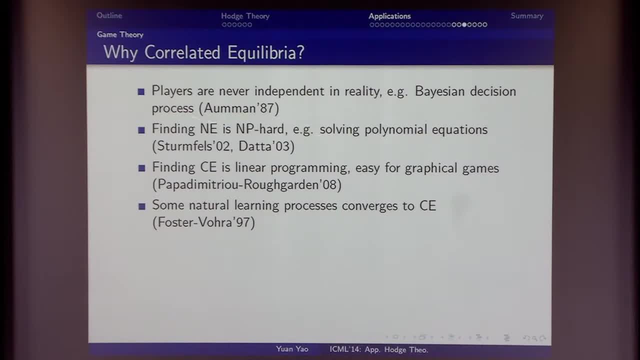 People mostly look at Nash equilibrium, But in reality Forman suggests correlated equilibrium, Because they think people never decide. They make decisions fully independently in reality. So players' decisions may be influenced by its relatives and maybe its close friends, And so decisions or process may happen in the reality. 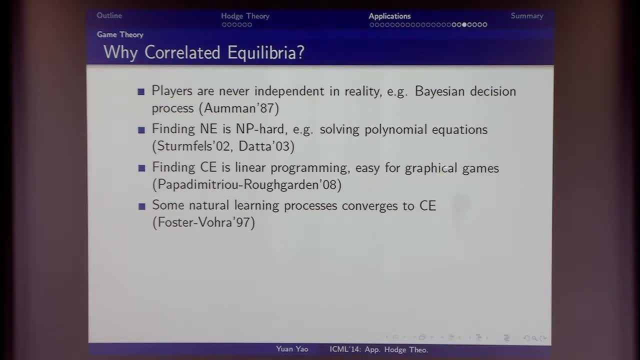 So he suggests correlated equilibrium may be more suitable to study than this kind of Nash equilibrium fully independent case. But another reason is finding Nash equilibrium. Nash equilibrium is notoriously NP-hard. You need to solve polynomial equations. But if you just look at correlated equilibrium, finding a single correlated equilibrium is a linear programming relatively easy. 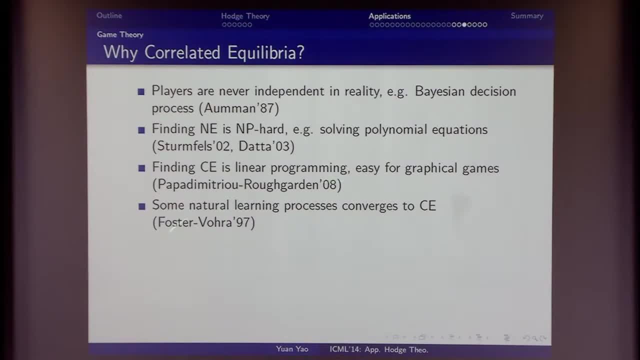 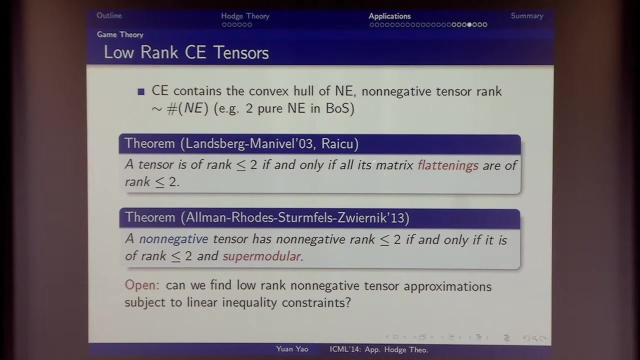 Especially for graphical games And some natural learning process may converge to correlated equilibrium but not the Nash equilibrium. So these kind of reasons suggest people to consider correlated equilibrium more than Nash equilibrium. But the question is: Can we benefit from this kind of situation to see whether we can find the Nash equilibrium through this kind of structure? 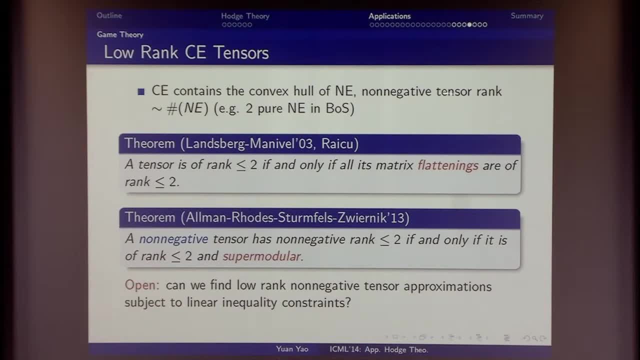 Actually correlated equilibrium contains the convex hull of the Nash equilibrium. It's a non-negative tensor, rank 1 or rank 2 or more rank, depending on the number of Nash equilibrium in the set Largely scale in that number. But if a tensor is rank 2, then we know if, and only if, all its matrix flattenings are rank at most 2.. 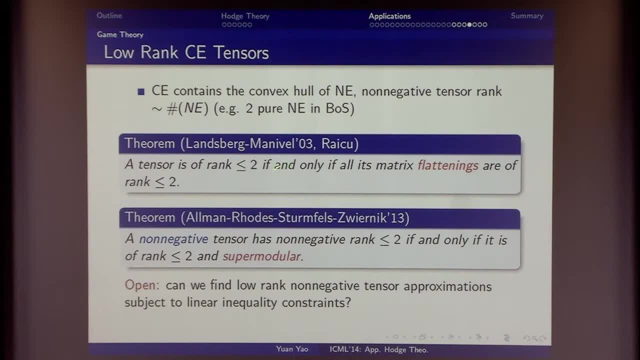 So that means if you have a tensor at most of rank 2, you can easily just look at all its matrix flattening. Use matrix linear algebra like SVD to find such low rank tensor. However, if you look at a non-negative tensor, if it is as non-negative at rank at most 2.. 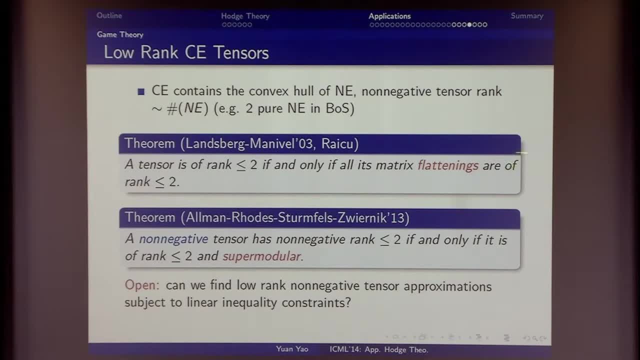 Then you need both rank at most matrix, flattening rank at most 2 and supermodular. So this situation makes things harder. So can we find the low rank non-negative tensor approximation, given the linear inequality constraints? This is a kind of interesting question, suggested from 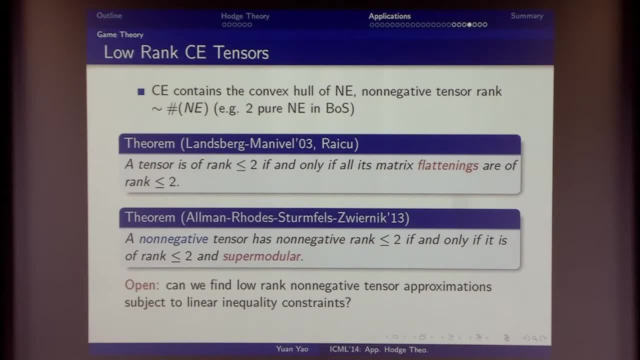 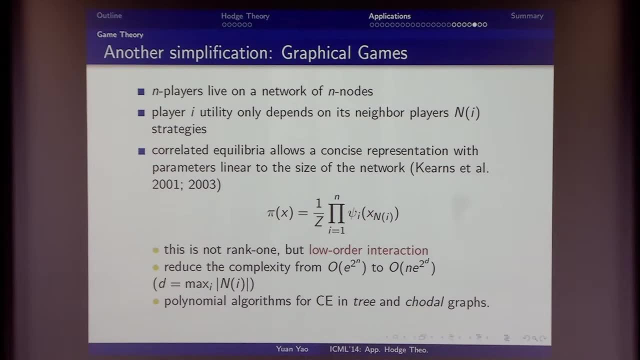 If we look at Data, if we look at the data from this point of view, And another kind of direction for simplification of games is kind of graphical games- Means that we have a N player live on the network of N nodes And every player has utility only depend on its neighbor players. 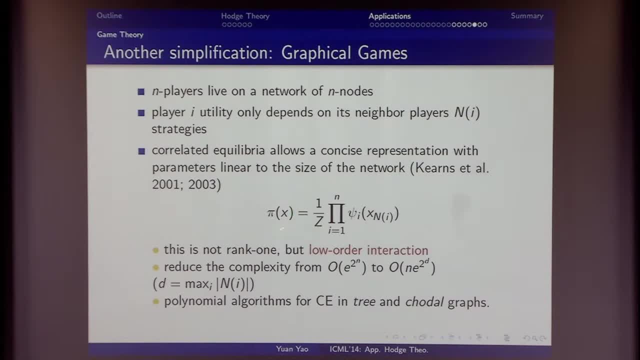 This kind of constraint leave you a joint distribution factorization In the In this product way. it's not rank 1 factorization but low order interaction depending on the neighborhood size. So you basically can restrict your factor. each factor on the click. maximum click on the on the on the graph. 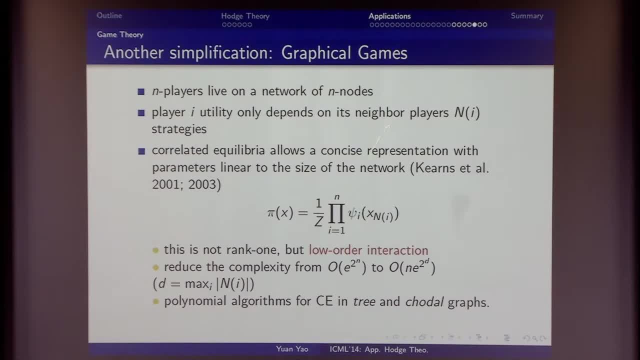 So this one can reduce from the double exponential complexity of representation for this joint distribution to double exponential To enable maximize neighborhood size. And we hope to have a polynomial, correlated polynomial algorithm to find correlated equilibrium in some simple graph like trees and total graphs. So this kind of a structure, and no matter which one before, 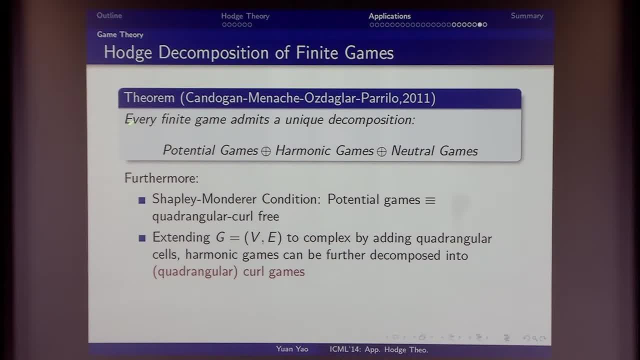 And we find actually Pablo Pereiro recently suggest every final game and makes a unique. decomposition means The data We Map to the graph flow always decompose into as a potential game and the harmonic game and the risk neutral game districts. neutral game means every player can translate their utility by a constant and doesn't change their relative preference. 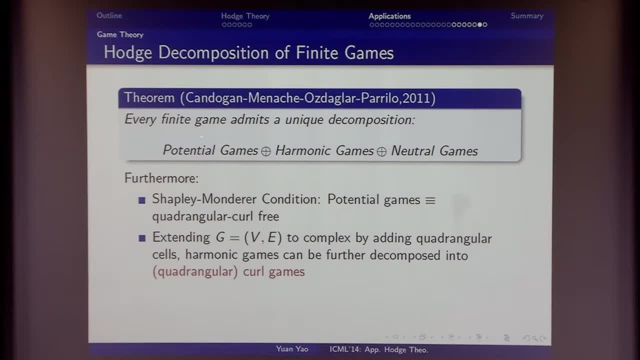 But this one will lead to this: neutral games, but the other two will be much more important because of potential game and harmonic game. This might be easier to solve in literature. So, if you consider the Sharpton Mandela condition, game theory, actually every potential game, if, and every game is a potential game if, and only if, every triangular cone equals to zero vanishes. 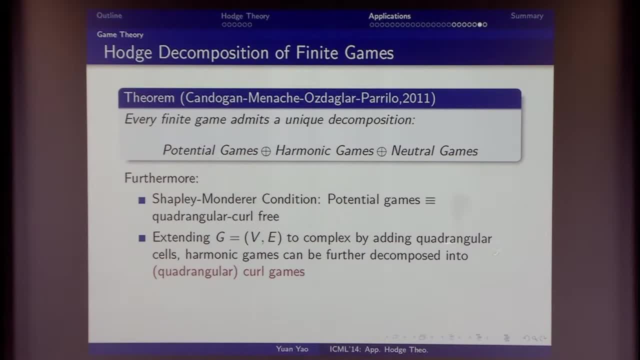 So you can further decompose this potential game by adding quadrangular cells rather than triangular cells. in this game case, harmonic game can be further decomposed into quadrangle And that way you can localize the game and make the harmonic part much more localized, and this may give you another kind of a way to look at that game. 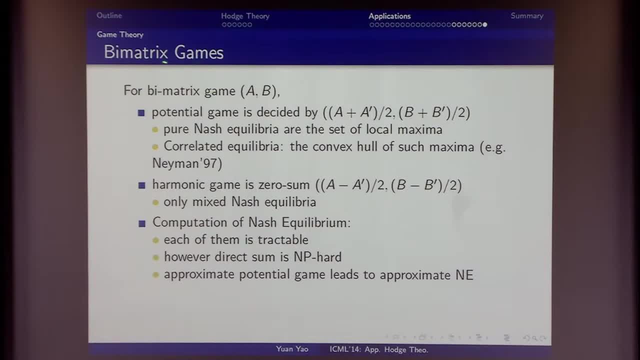 The composition. So, in particular, if you look at a biometrics game like the example we propose in the beginning for the battle of sex, such game always decided by a potential game, by the symmetric part of this, by matrix one, and the harmonic game is decided by the skew symmetric part, and these parts are very 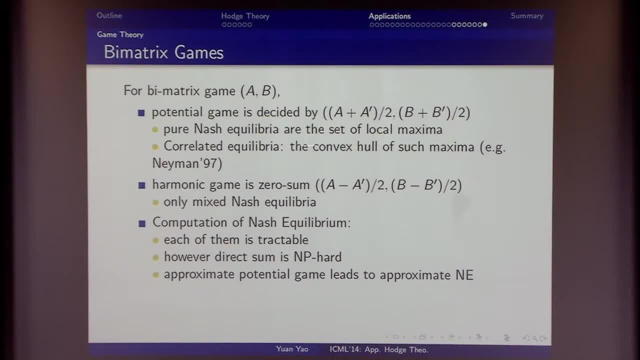 easy to solve because the symmetric part, all the pure Nash equilibrium just decided by the local maximum and correlated equilibrium, will be the convex hull of such maximum and the harmonic game. actually, no pure Nash equilibrium here, only mixed Nash equilibrium. and what's the benefit if you decompose game into this way? because if each of them the potential or zero sum, each of them, 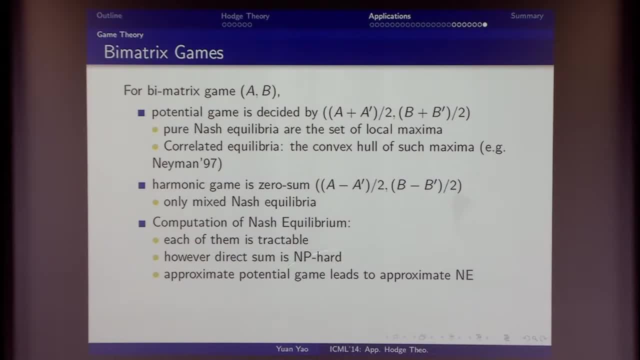 will be tractable. however, their direct sum is not tractable, is very NP hard in the worst case. but if your game is close to a potential game, then you can easily achieve the approximately Nash equilibrium in this case. but on the other hand, we don't know if it is close to harmonic. 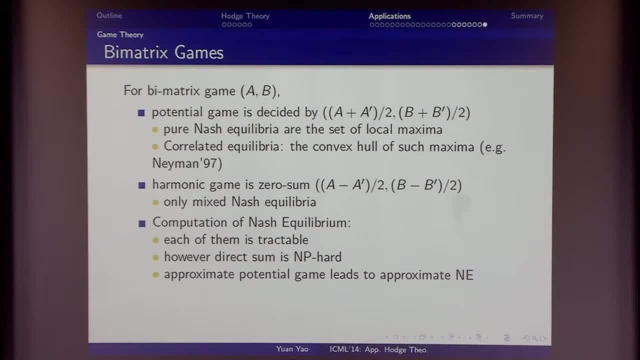 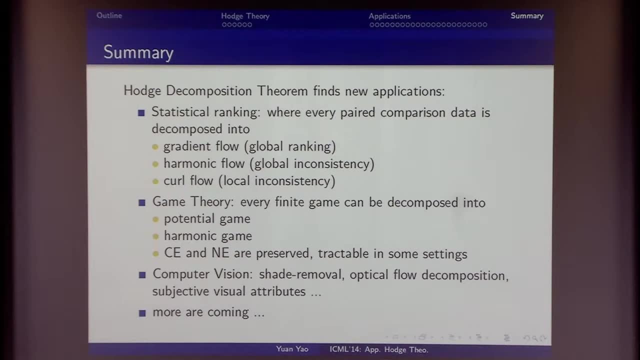 game. what's the usage, what's the benefit can we benefit, we can obtain from such a decomposition? so this kind of application for game theory and so, as a summary, I basically mostly cover focus on the statistical ranking, and every such pairwise comparison data can be mapped to gradient flow, harmonic flow and the curl flow and the comparably in game theory you get a. 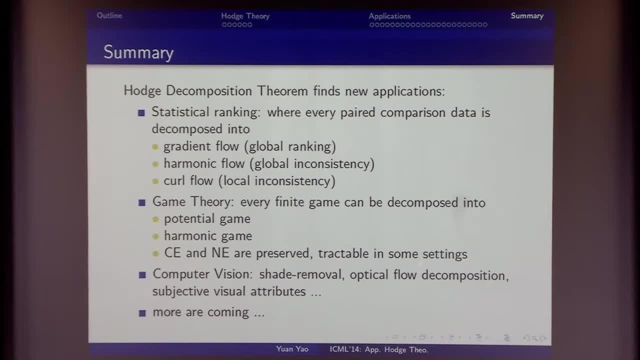 identical section that is shown why what happen in a semi-quad are here, so it can be in the form of sequential game and harmonic game. why curl doesn't appear? because you use Nick a triangle click suggests by, originally by fellow parallel. but if you look at a quadro, angle cells and map them and 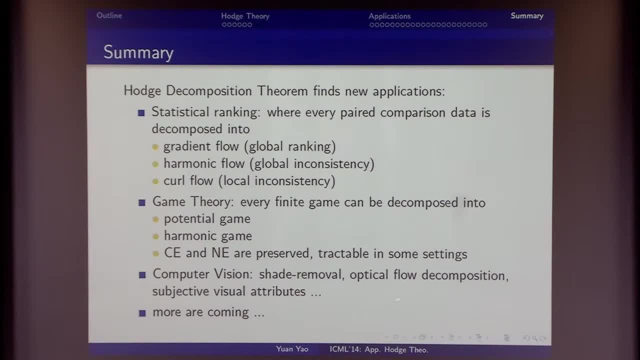 put them into the south, some famous Oh complex, and you get a quadrangle curl flow. so this kind of think I may help you to find the equilibrium and we some settings that you can get tractable and either application in computer vision. we hope to find more in the future, so hopefully, 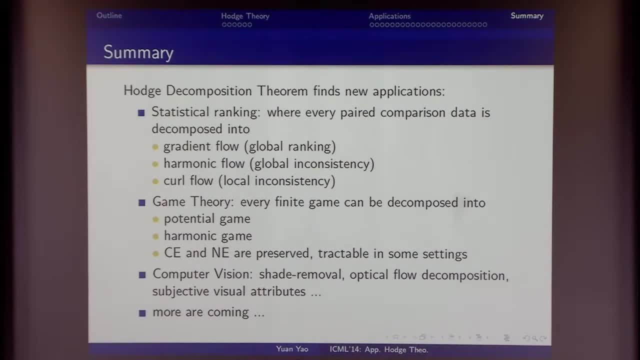 this kind of introduction does not make you to feel too much boring with Hodge decomposition. personally, I like this structure very much, although it's simple, but it appears in from very deep algebraic topology to very simple linear algebra. so thank you for your listening. and these are my collaborators and 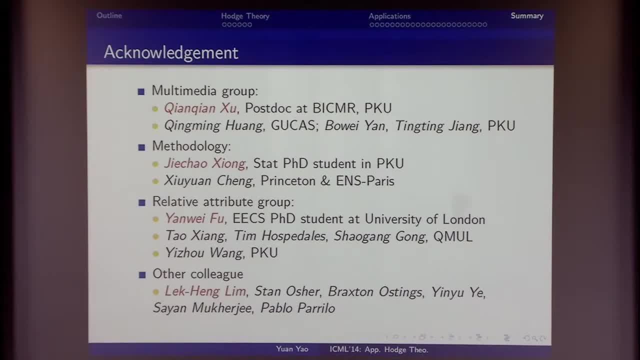 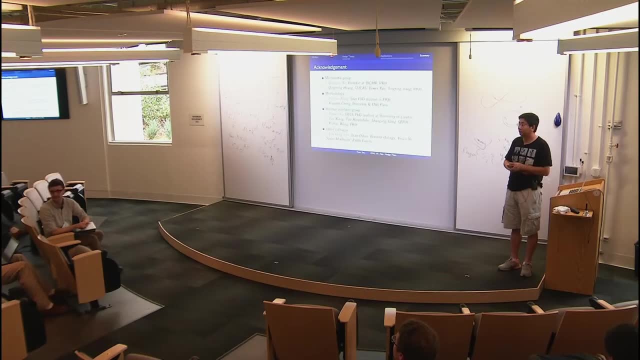 friends, any questions? a question: yeah, so when you do the? so we want to get the harmonic free ranking? yeah, is it simply a matter of just adding all triangles? yeah, so when you want to get the harmonic free ranking, is it simply a matter of just adding all triangles? 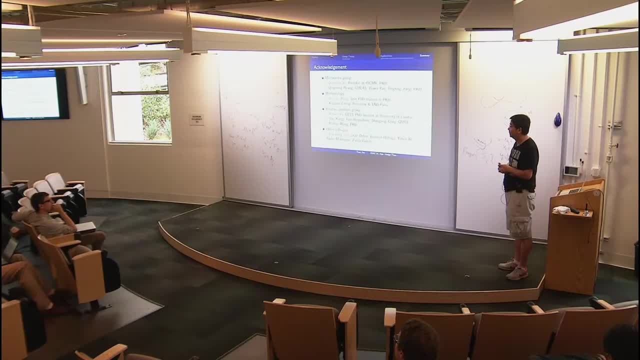 yeah, so when you want to get the harmonic free ranking, is it simply a matter of just adding all triangles? yeah, so when you want to get the harmonic free ranking, is it simply a matter of just adding all triangles? actually, the original suggestion by Pablo is he only used triangular faces. actually he put because every player can.